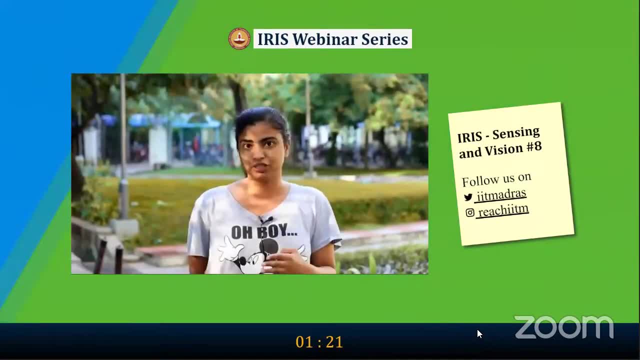 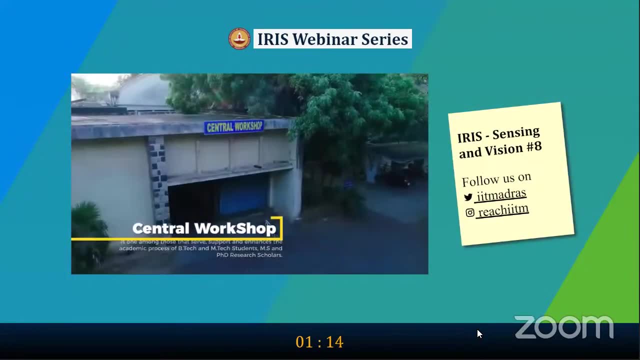 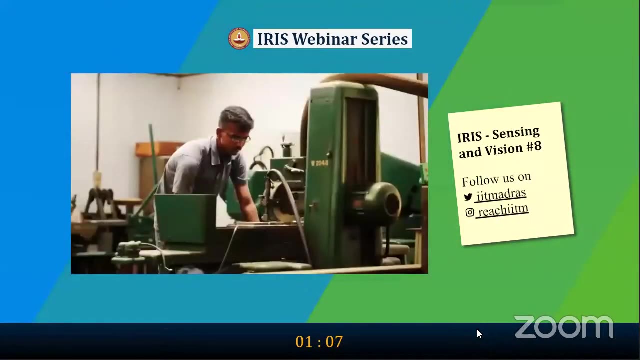 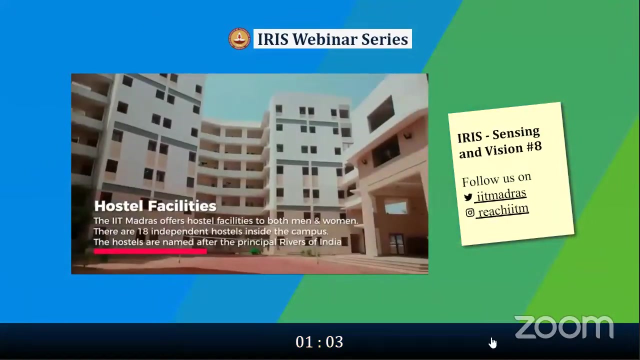 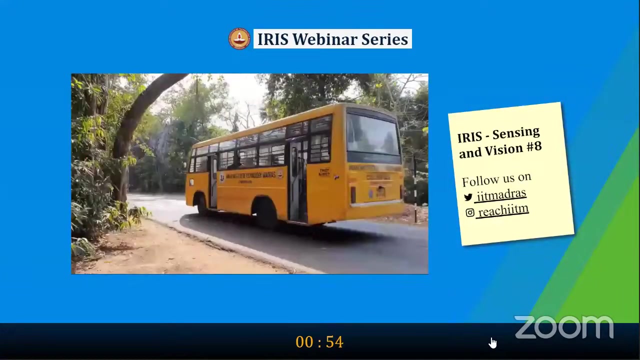 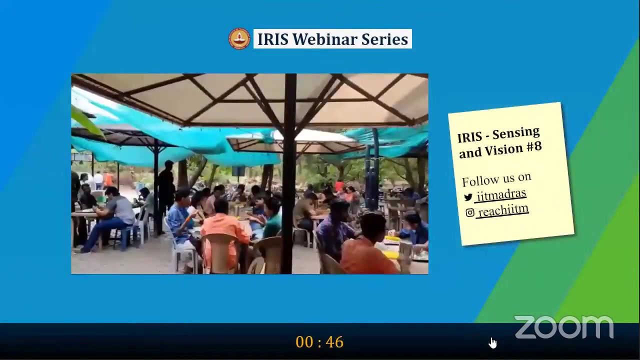 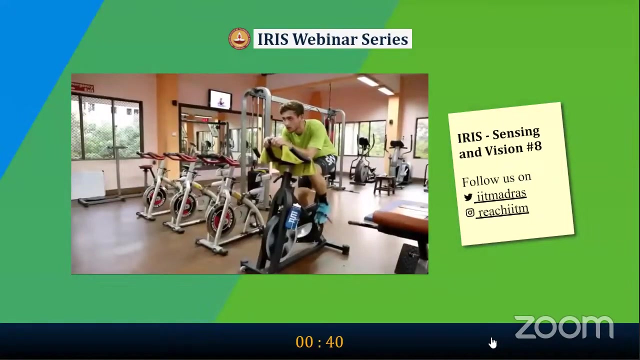 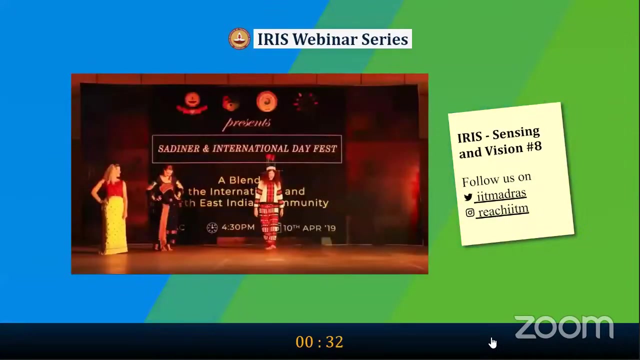 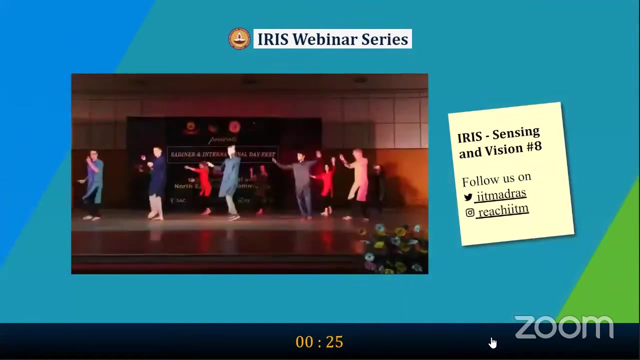 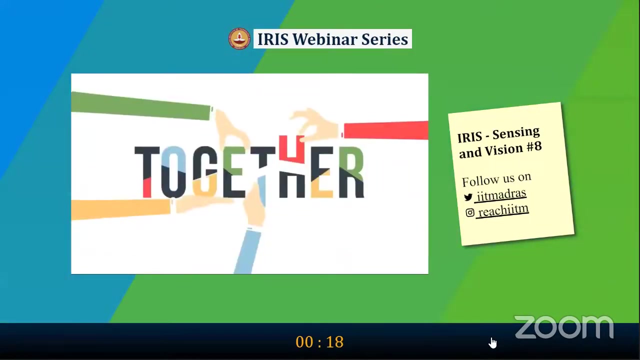 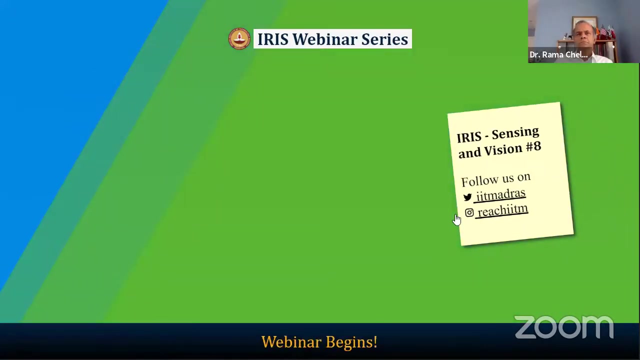 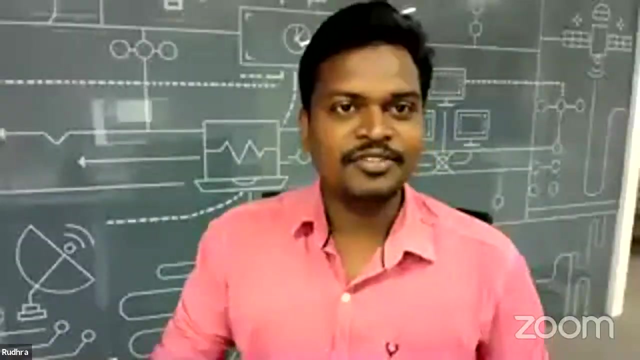 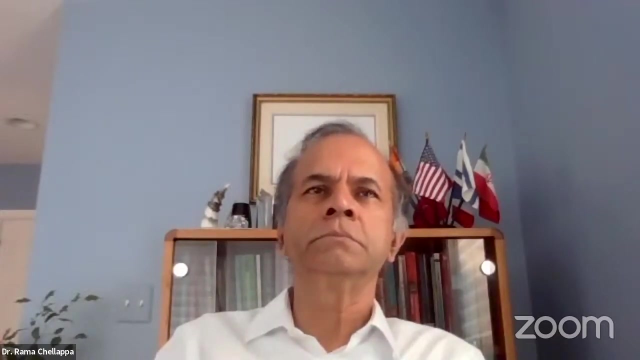 Because you have the time and also opportunity to explore each and every thing, Thank you. Thank you for the wonderful video, Shivram. I think we can get it started. Good evening and a very warm welcome to everyone. We appreciate you being here with us today. 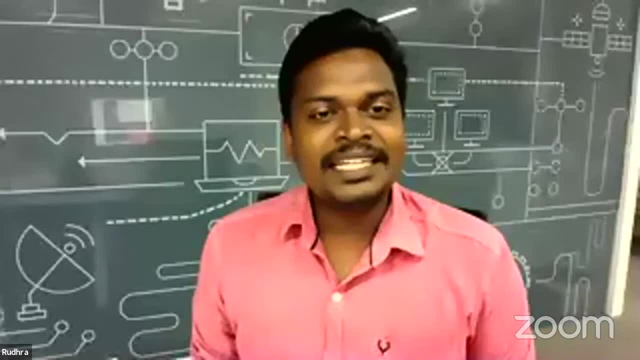 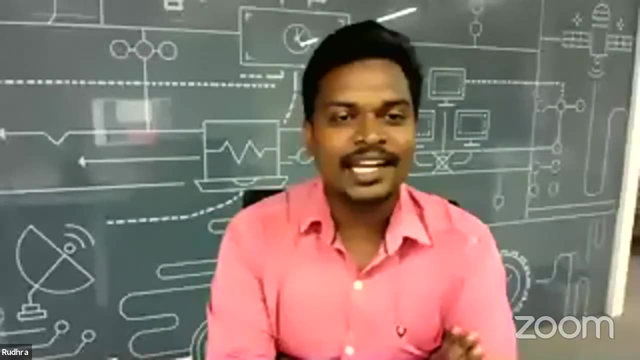 And it's nice to see you all here again. So, as I've been telling in the previous webinar that the IRIS webinar series is gaining momentum in the public domain, And it's my pleasure to happily share that, we have already crossed thousands and thousands of registrations and participants. 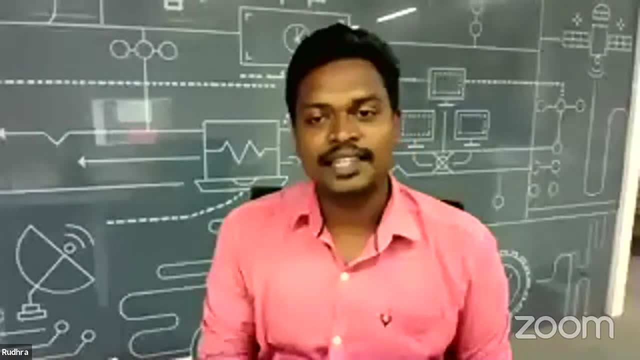 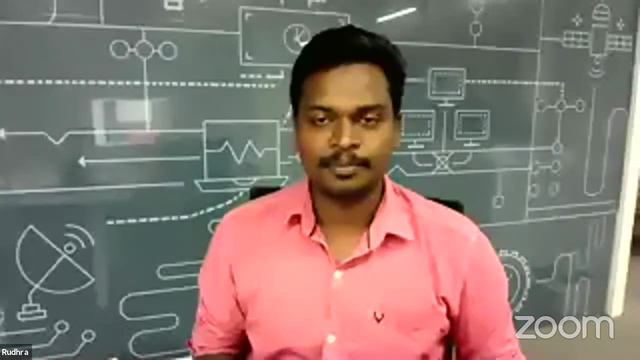 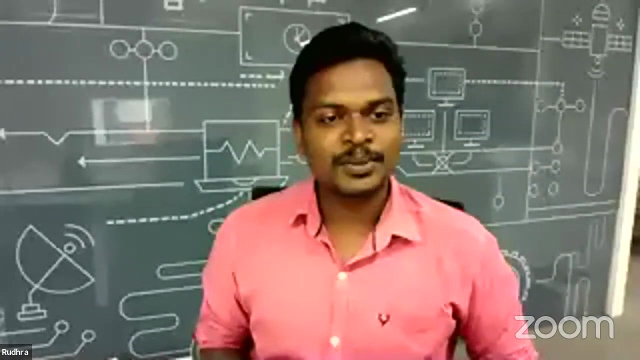 So the main idea behind these webinars is to showcase the innovative research being generated at IIT Madras to various stakeholders like researchers, industrialists and policymakers. And yes, we are here again And it's our pleasure to present the eighth webinar, which is computer vision, in the IRIS webinar series under the cluster sensing and vision. 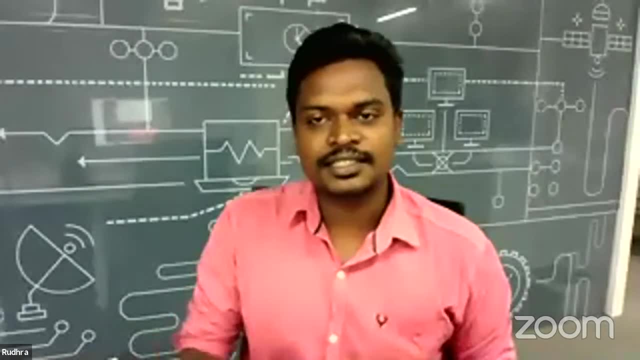 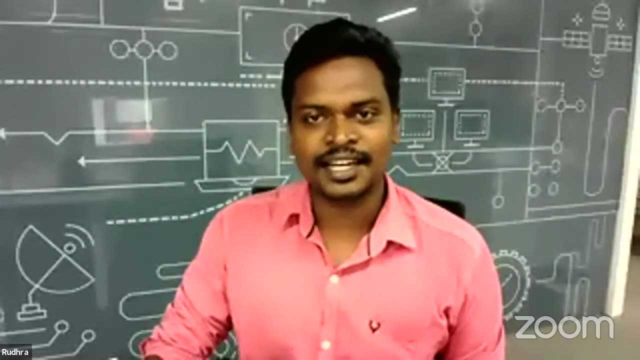 So the research initiative under the computer vision technology project is led by Professor AN Rajgopalan. To say a few words about Dr Rajgopalan, So he's a satellite technology chair professor in the department of electrical engineering at IIT Madras. 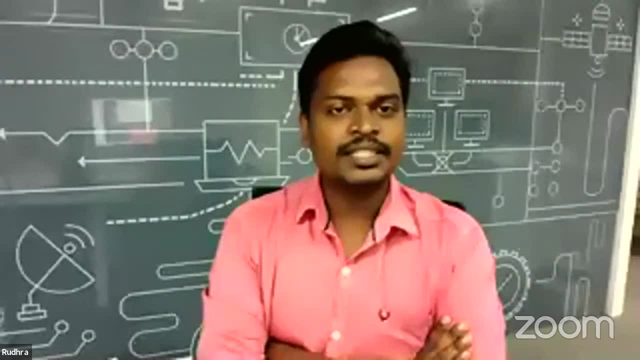 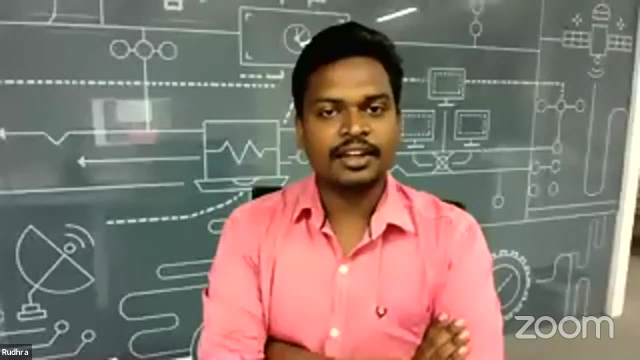 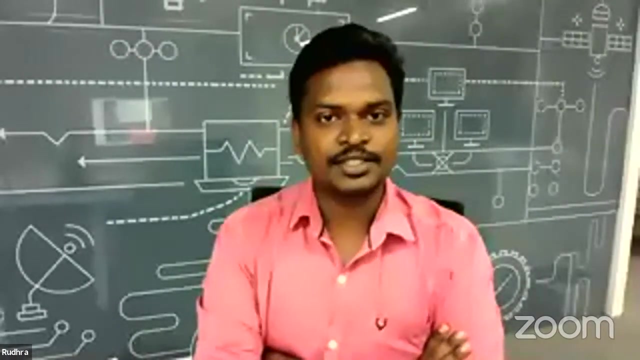 And also head the image processing and computer vision lab. So he's a fellow of the Indian National Academy of Engineering, fellow of the Alexander O Humboldt Foundation, Germany, and also the fellow of the Institution of Electronics and Telecommunication Engineers. So he has served as the Associate Editor of IEEE Transactions on Pattern Analysis and Machine Intelligence from 2007 to 2011.. 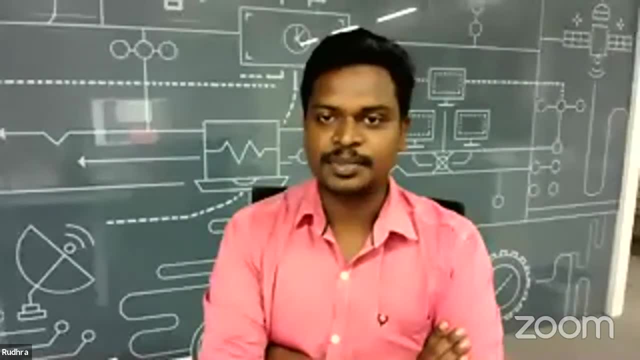 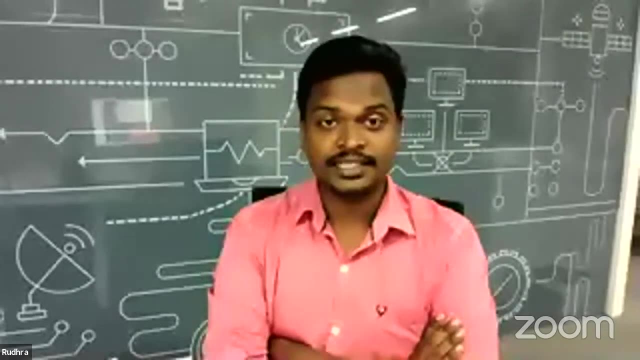 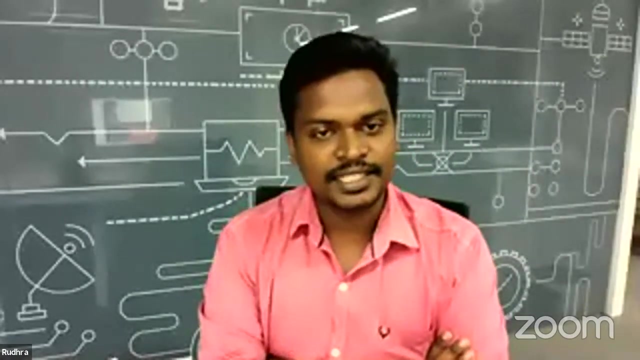 And also as the Associate Editor of IEEE Transactions on Image Processing from 2012 to 2016,, and also as a Senior Area Editor for IEEE Transactions on Image Processing since 2016.. So he is the recipient of the DAE SRC Outstanding Investigator Award in 2012.. 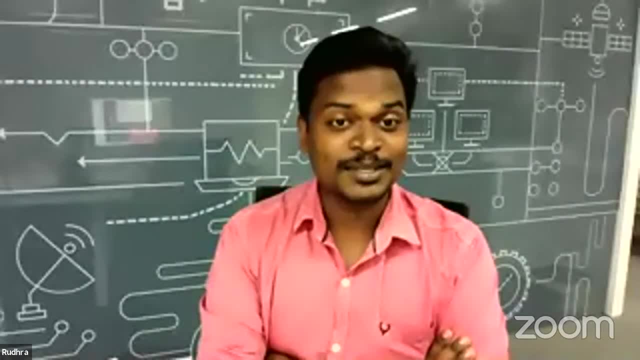 So the VASBIC Industrial Research Award in 2013 and the DEMED Career Institute Research and Development Award from IIT Madras in 2013.. So the VASBIC Industrial Research Award in 2013 and the DEMED Career Institute Research and Development Award from IIT Madras in 2014.. 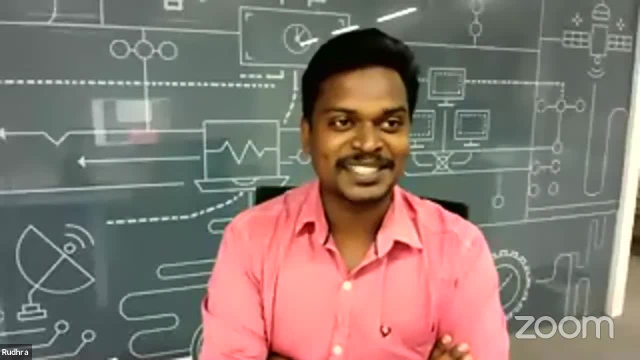 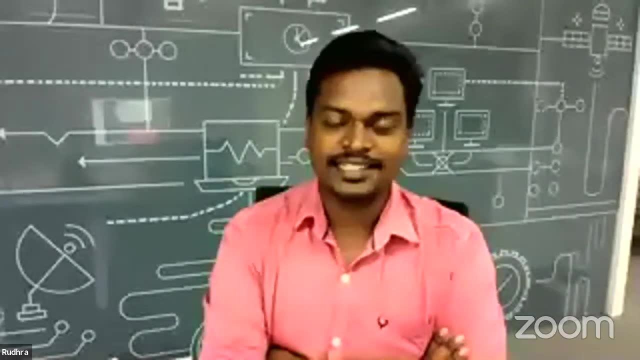 And the Google India AI ML Faculty Research Award in 2018.. It goes long and long. His research activities are funded by MHRB, BST, DAE, DRDO, AFRL and KLA Tenka from USA, Google India, Aroob from USA, among others. 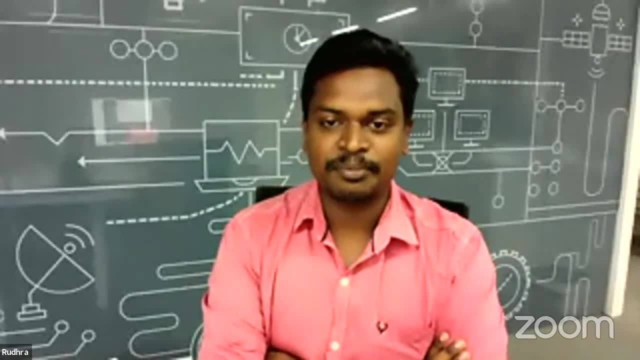 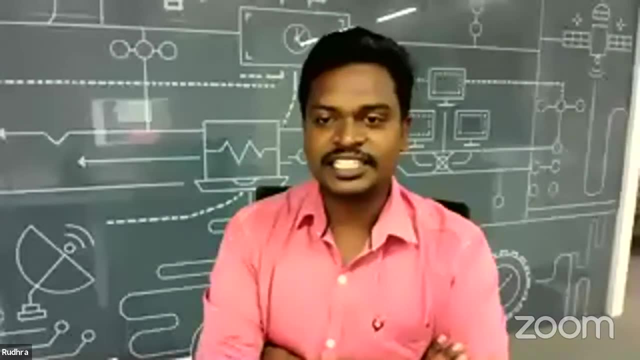 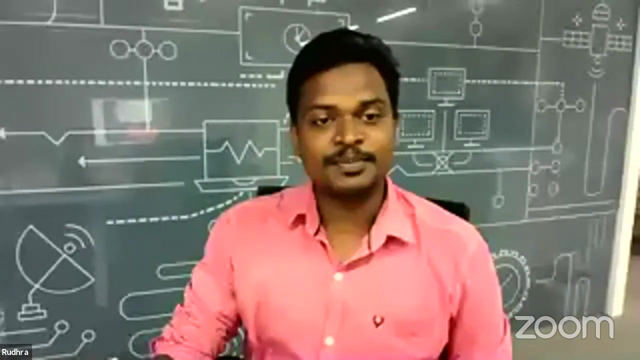 So he had held visiting positions at the University of Maryland Technical University of Munich. So Professor Raj Gopalan's current research interests include recovering shape from X, image restoration, Image forensics, underwater imaging, Deep learning, Multi-Modal Learning and sport analytics. 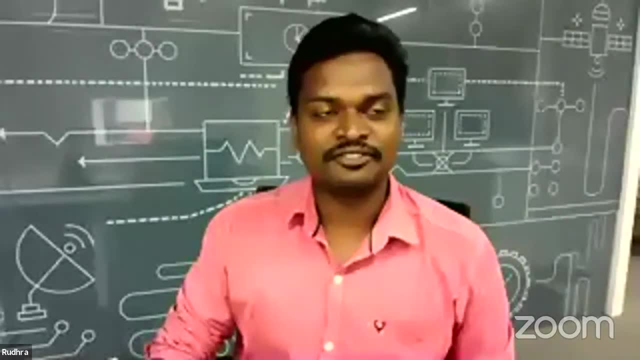 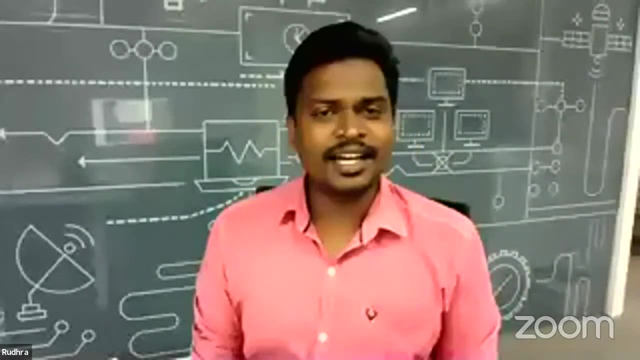 So joining Professor Raj Gopalan as a speaker today's webinar. Thank you, sir. So we also have Dr Rama Cellapa has joined as the moderator. Well, he is a Bloomberg Distinguished Professor in the Department of Electrical and Computer Engineering andع. 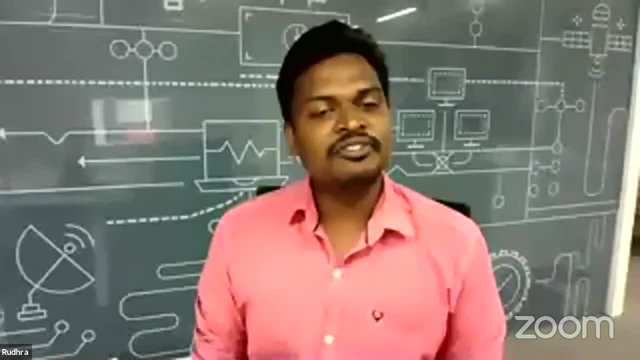 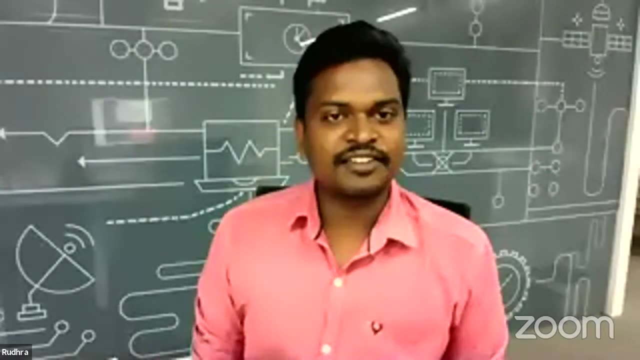 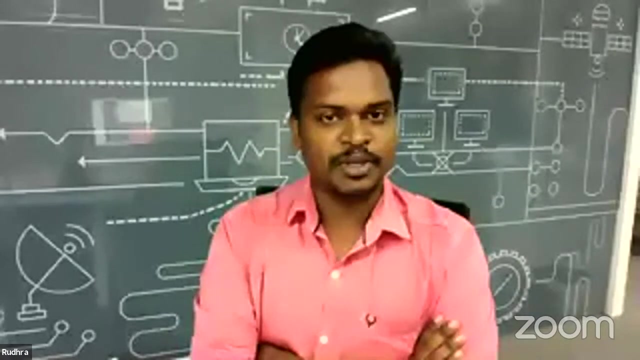 Biomedical Engineering at Johns Hopkins University. So before joining JHU in August 2020, he was a Distinguished University Professor at Minta Martin, a Professor of Engineering, a Professor in the EC Department and the University of Maryland Institute of Advanced Computer Studies at UND. 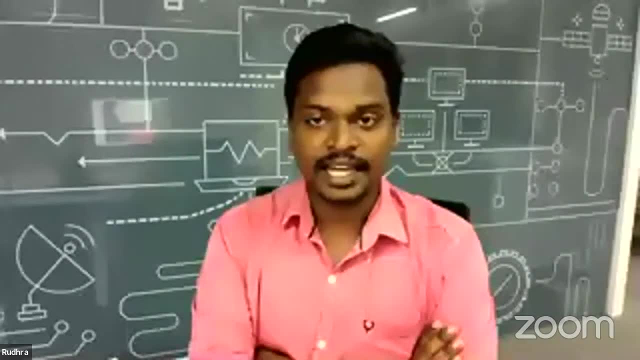 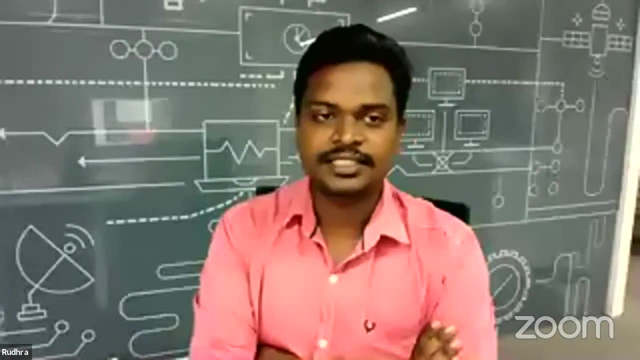 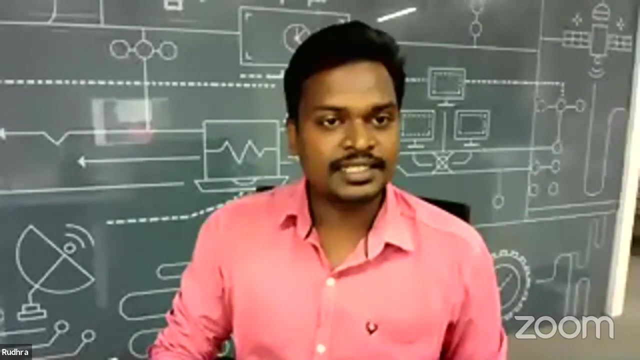 So he's a recipient of 2020 IEEE Jack S Kilby Signal Processing Medal. He's also a recipient of the KSFU Prize from the International Association of Patent Recognition. He also received the Technical Achievement and Meritorious Service Awards from the IEEE Computer Society. 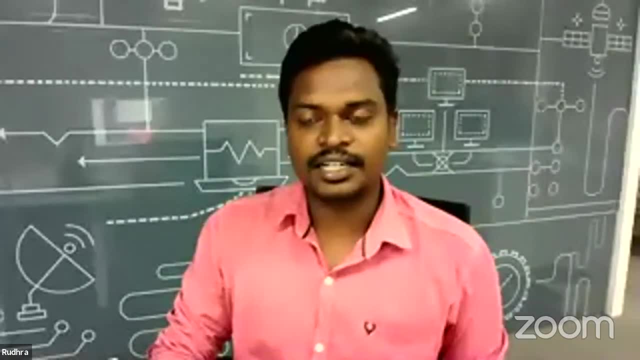 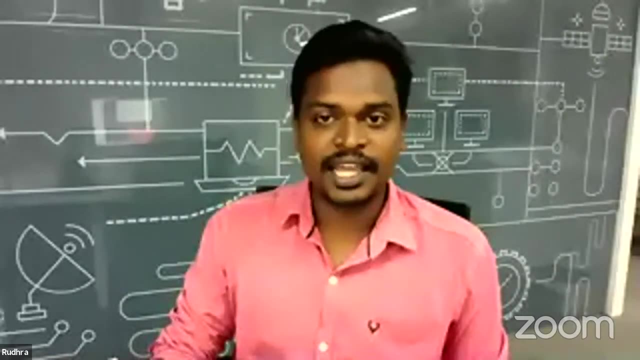 Recently he was recognized with the Inaugural Leadership Award from the IEEE Biometric Council. He's a fellow of IEEE, IAPR, OSA, AAAS, ACM and AAAI, So he served as the Editor-in-Chief of IEEE Transaction. 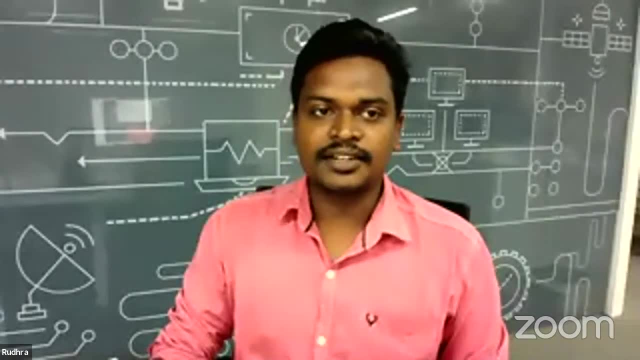 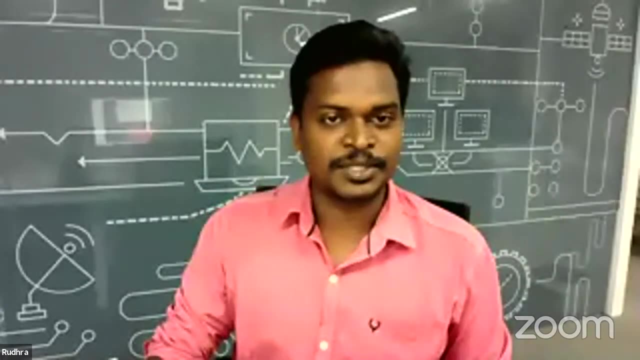 on Patent Analysis and Machine Intelligence. He has served as a General and Technical Program Chair for several IEEE International and National Conferences and Workshops. He's a Golden Co-Member of the IEEE Computer Society and served as the Distinguished Lecturer of IEEE Signal Processing Society. 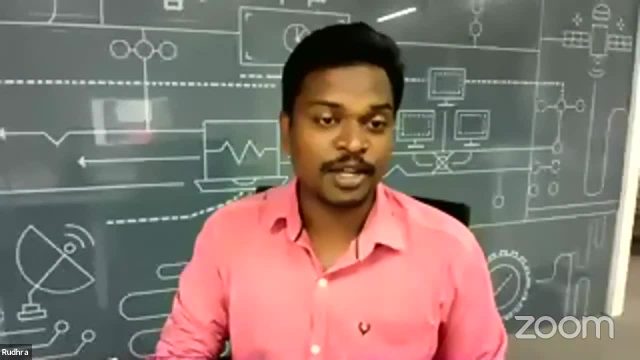 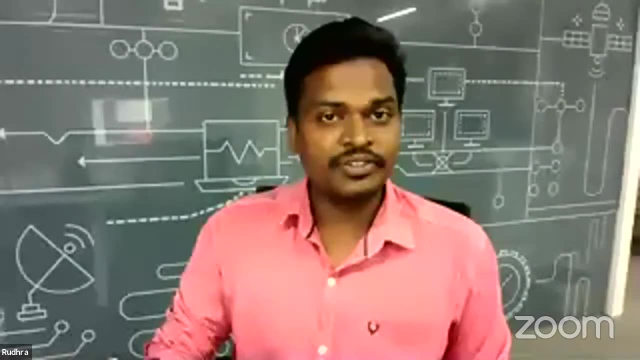 He served as the? I inaugural President of the IEEE Biometric Councils too, So Professor Chalapa's current research interests are computer vision, machine learning, artificial intelligence and signal and image video processing. So it's my pleasure to invite you both to this session, Professor. 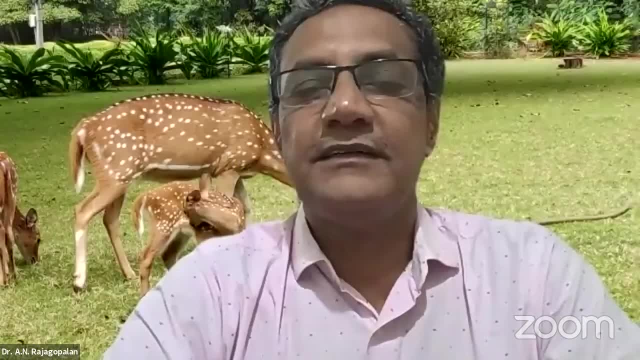 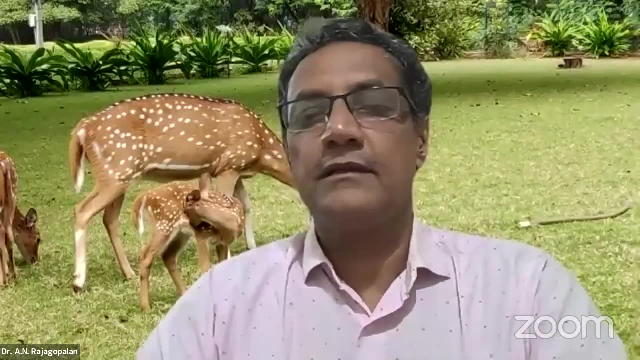 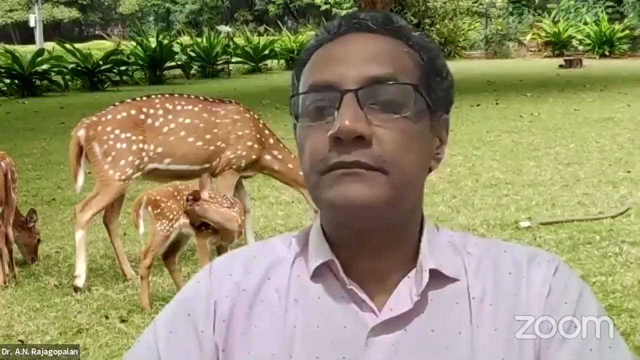 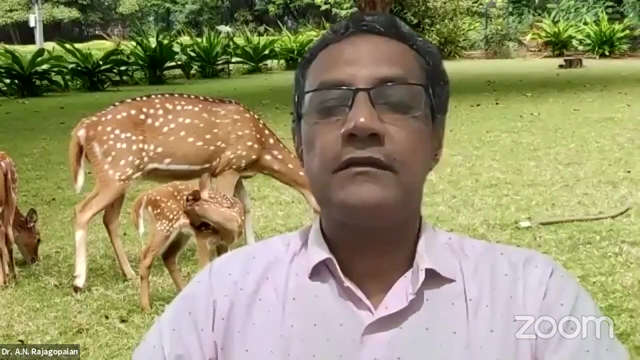 Over to you, Dr Chalapa. Thank you, Professor Chalapa. Yeah, Hi, Yeah, you can leave the session. The floor is yours, Okay, Oh, thank you. All right, Roger, we are all waiting to hear from you. 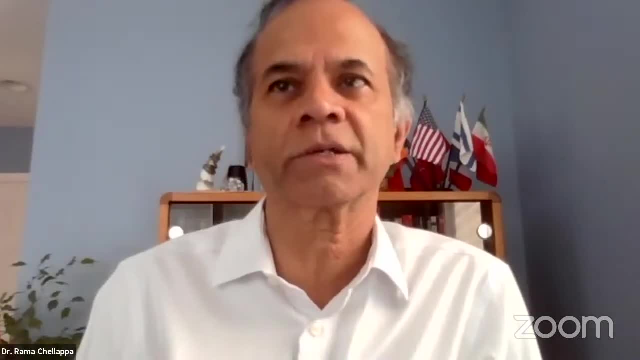 I guess you're going to give a presentation and those in attendance can put your questions in the chat box, And so it's about 30 minute presentation, is it Right? Right, It's about 30 minutes. Yeah, Yeah, Go ahead please. 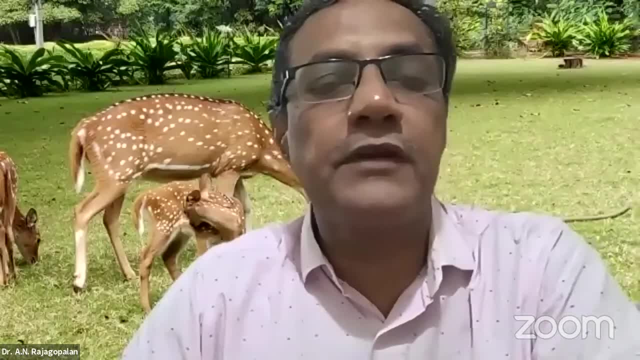 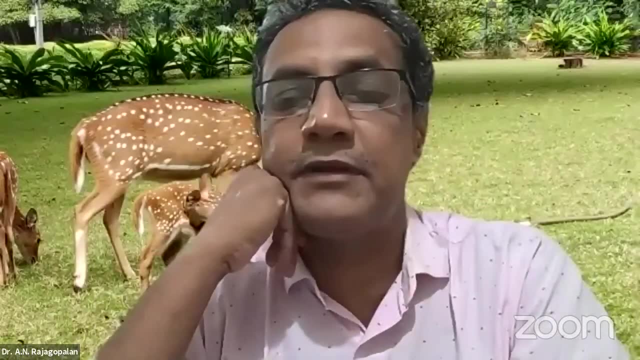 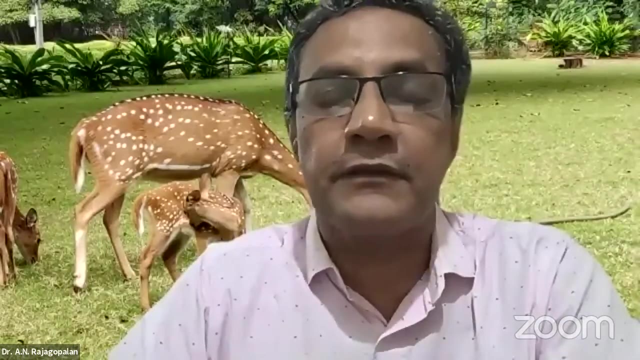 Thank you. Thank you, Professor Chalapa. This is Raja Gopalan. I am a faculty in the Department of Electrical Engineering at IIT Madras And I head the IPCV lab at IIT Madras, And I am here to share a research initiative on this prospective Center of Excellence in Computer Vision. 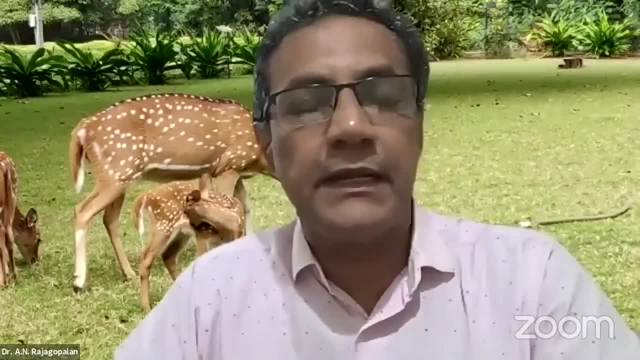 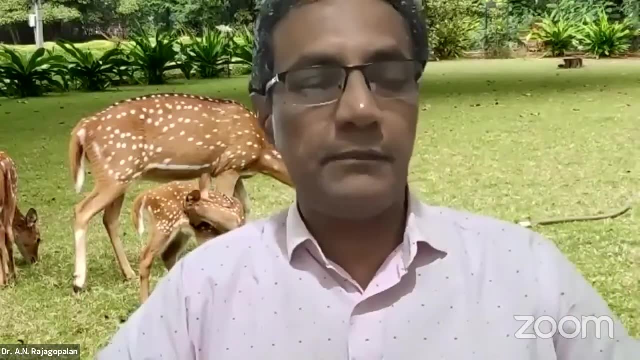 And I will try to move on to the next slide. I mean, are you able to see my slide, by the way? No, we don't. I don't see your slides. Okay, Then, maybe, maybe, Okay. Let me just start sharing it because, for some reason, 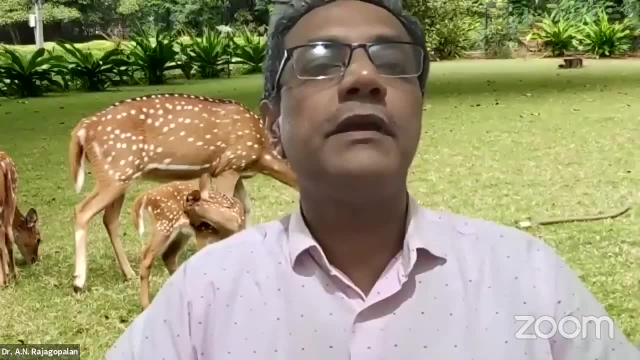 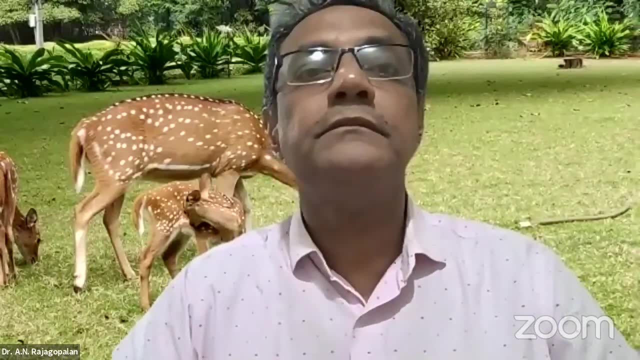 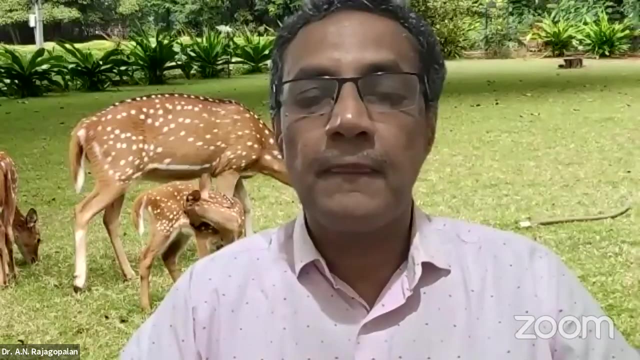 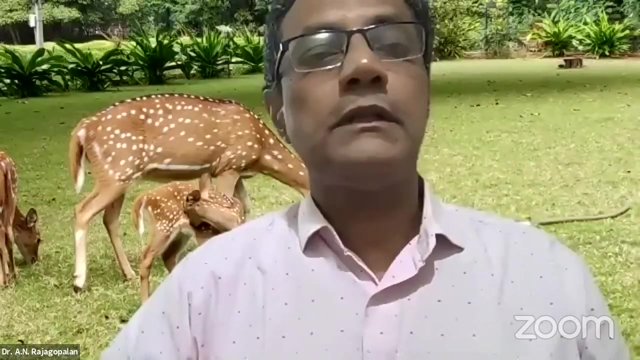 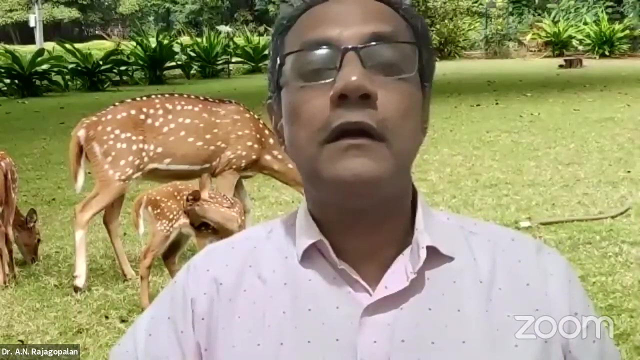 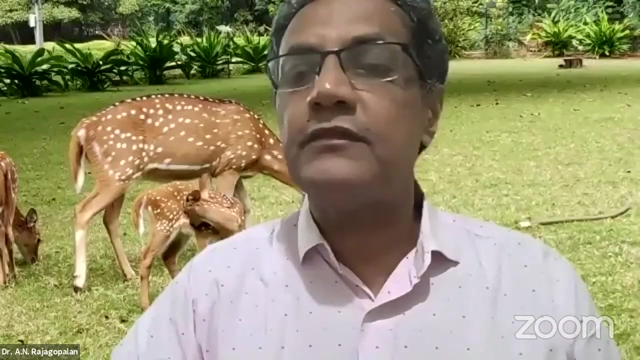 One minute. Okay, Let me see Just a second. Let me let me get this screen sharing going Clicking on the Zoom link. but for some reason, some reason, Do you need any help, Professor? Yeah, I mean my Zoom. Have you locked my screen or something? Because I'm not. 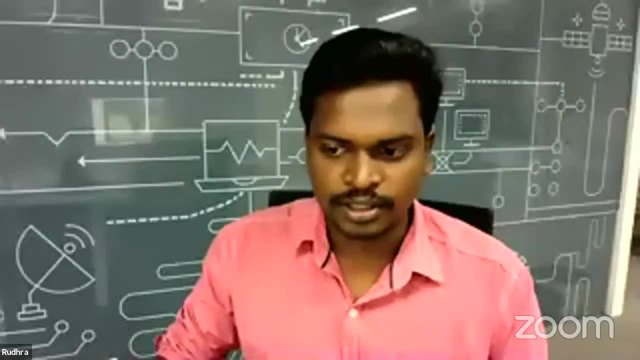 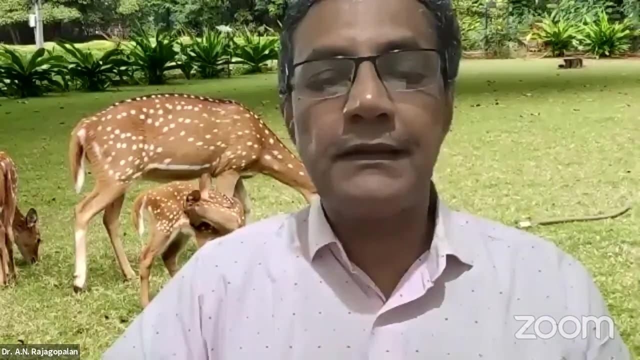 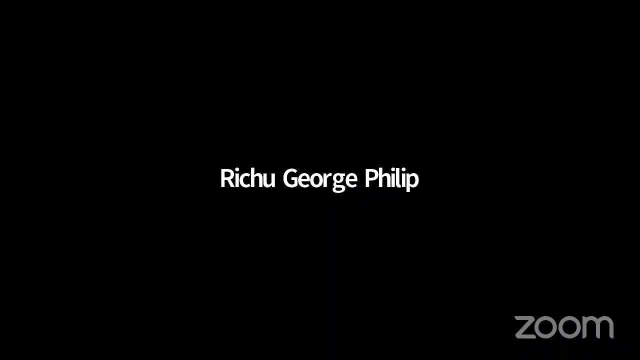 No, No, I'll just try to unspotlight you. Yeah, Naresh, can you please do that, Because my Zoom, when I click on it, it doesn't seem to do anything at all. Mr Naresh, Yeah, I have a remote spotlight. 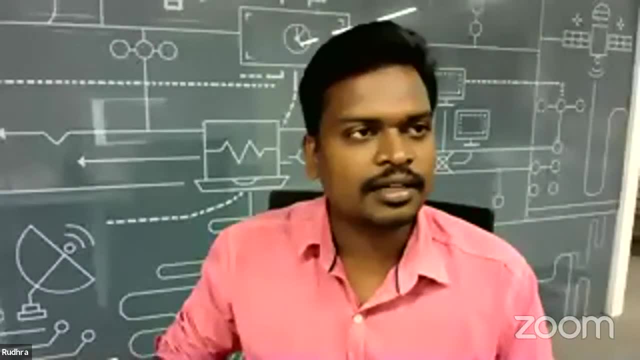 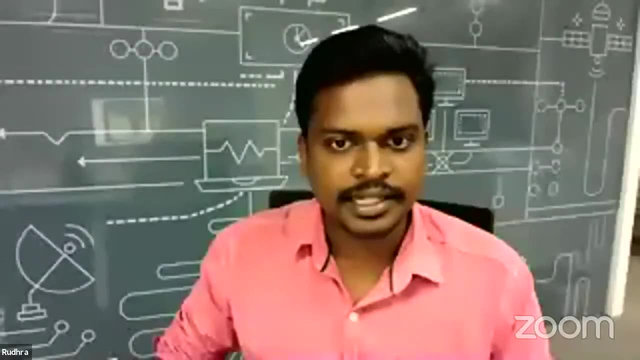 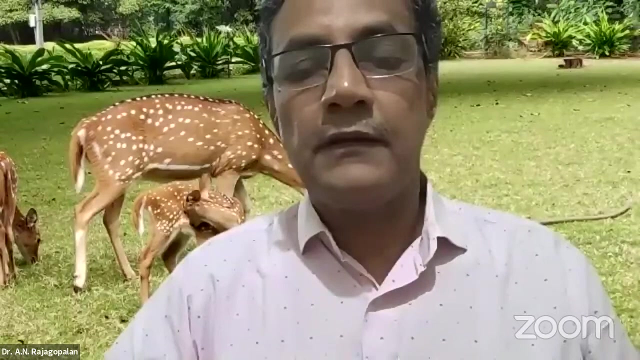 Okay, So I think just minimize, or else you can just minimize the screen and open it again. Okay, Can you share the click on share screen? No, when I click on the Zoom link, right, it doesn't come on. I mean, for some reason, when I click on the Zoom link. 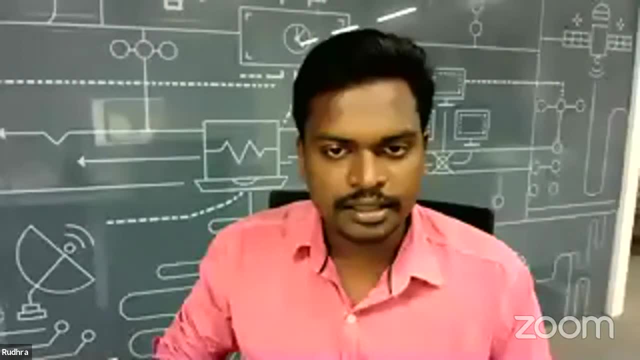 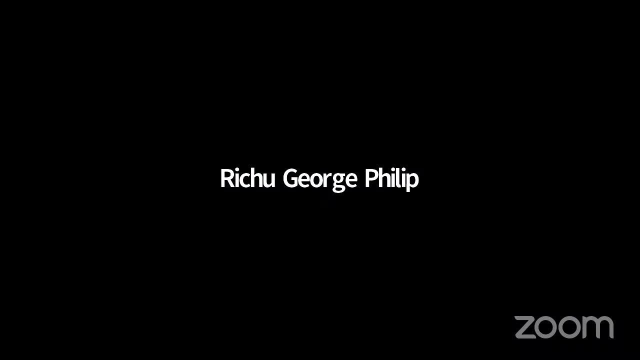 Are you trying to press in the screen from the, from a PowerPoint? No, no, no, no, This is supposed to be a Google slide. Okay, Google slide. Professor Raju, you could also email the slides to me. No, actually, right, it should work out. I'm just 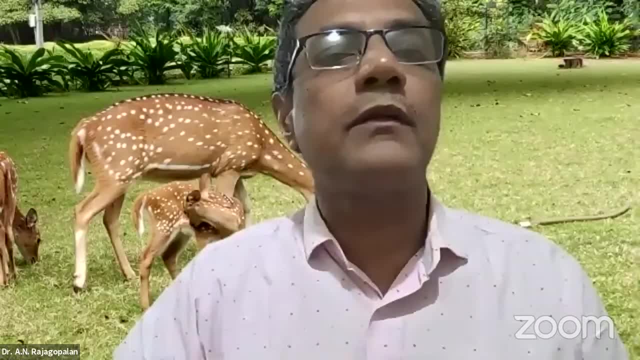 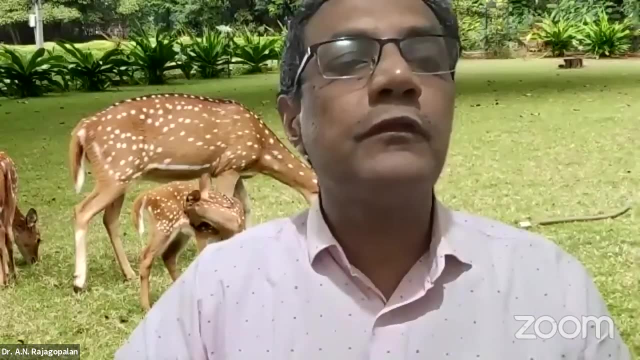 Okay, Okay, Okay, I think I think I'm fine. One minute, Just a second. Okay, I think I am there almost. Let me see, How do I, how do I get to the full view Then I think now everything will work out fine. 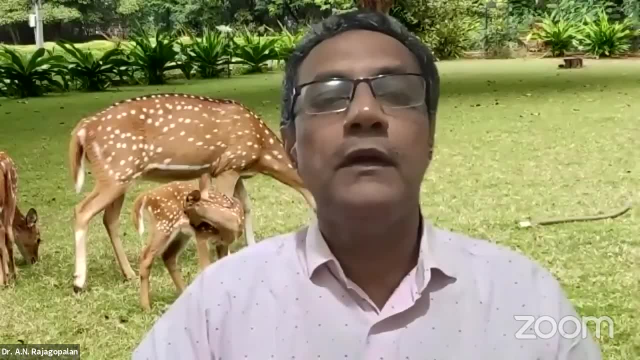 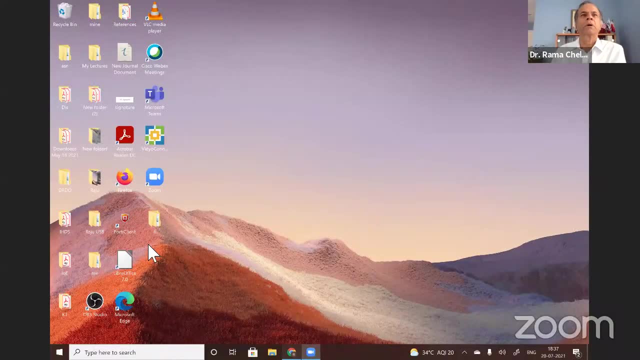 Okay, I think I'm kind of right, Good to go. So please tell me if you're able to see my screen. Yep, I think we. Yes, All right, All right, Very good. So I think now I should be done very quickly. 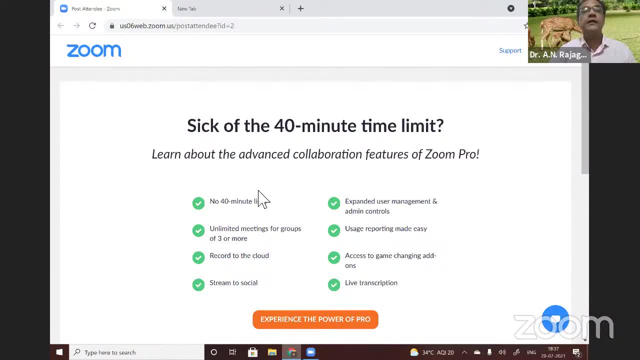 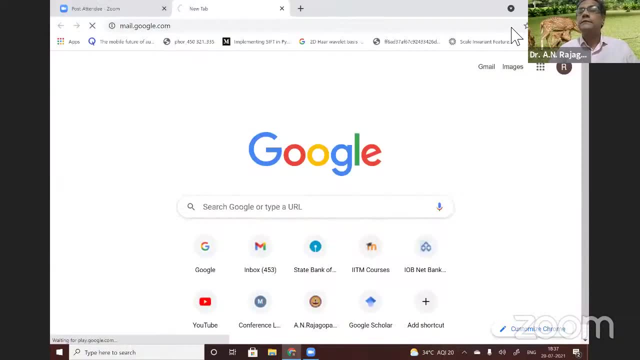 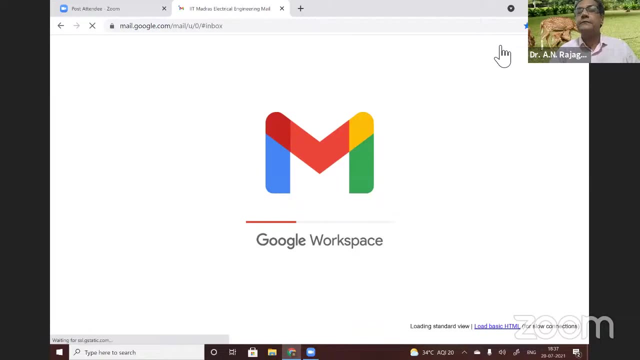 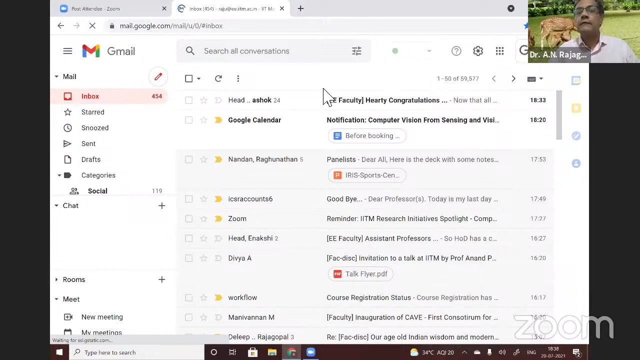 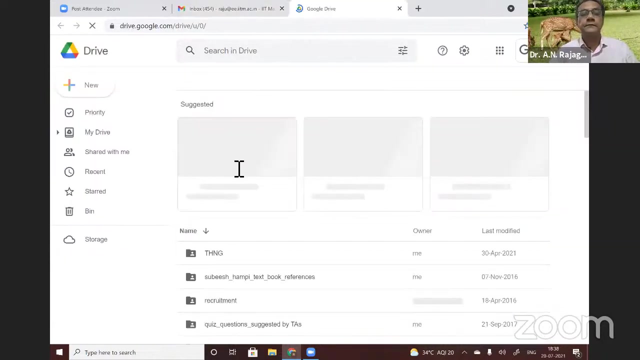 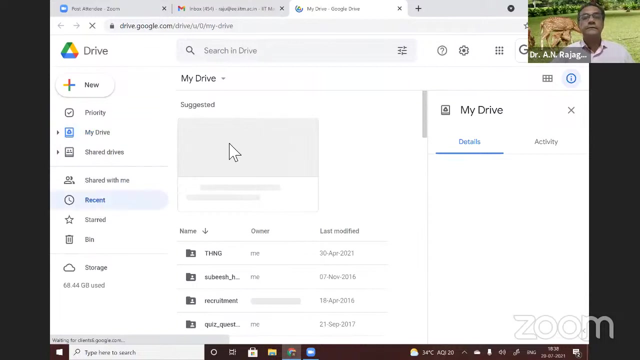 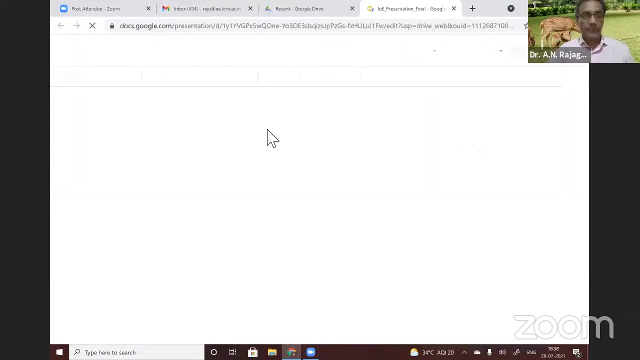 Let me just open my presentation Now. Sorry for that small delay. I had it on but I had to close it because we had to get the Zoom going. I had to go to my drive. All right, All right, I think we are all set now. 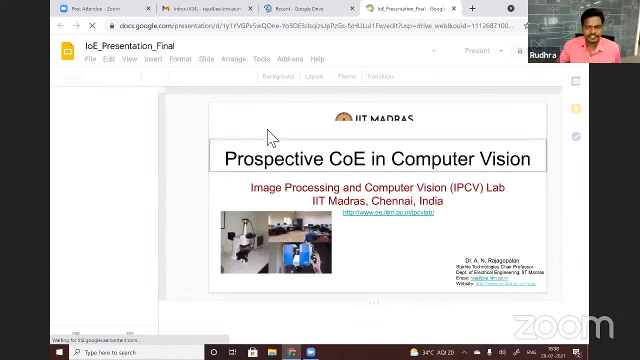 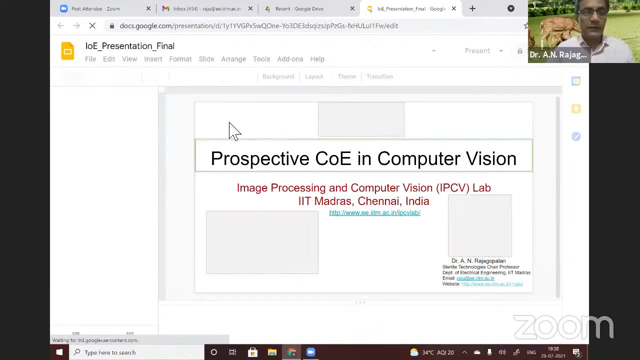 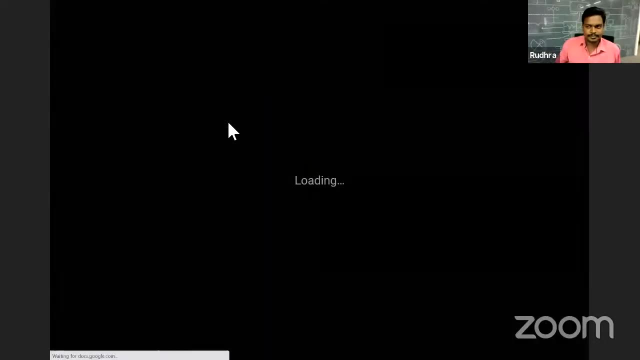 Okay, Now. are you able to see it full screen? Yes, Professor, All right. Thank you for bearing with me. Is it coming full screen yet? Yes, Just a second. I think it should load. All right, Now I can see it. Are you able to see it too? 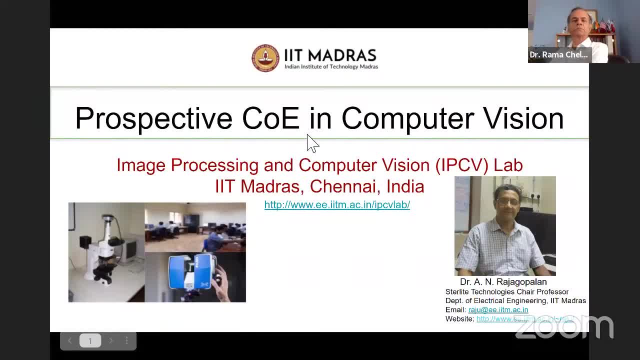 Yes, Yes, Go ahead. Okay, So let me start with my slide on acknowledgement, which is an acknowledgement to all my students who have been my research scholars, both the PhD and MS. These are all students, many from the past. some are ongoing students. 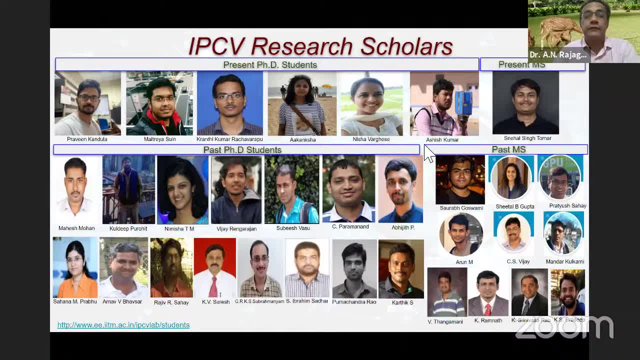 So, basically, these are the backbone of the lab, as is the case, I guess, with every lab around the world. And let me also mention that we have a very along the way. we would like to have a strong impetus for outreach, which also means that we are very keen about hiring young foreign faculty. 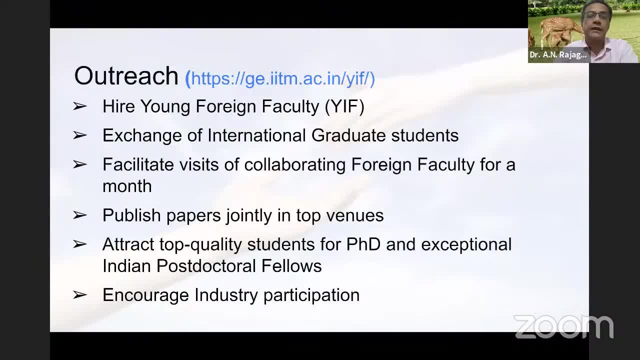 And, of course, I've shared this link out there, which you can actually click on later for those of you who want to understand how this entire thing works, because I don't have the time to go to the exact details of each of these mechanisms. 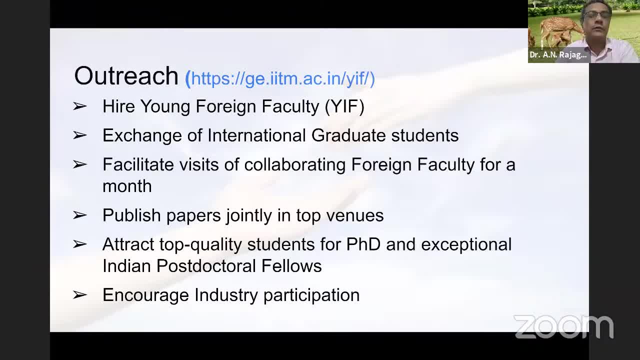 But just click on the link and you will know what information you want out there. And then, of course, we also want to encourage international exchange of international international grad students, facilitating foreign faculty visits, maybe for a month or so, or even more if needed. 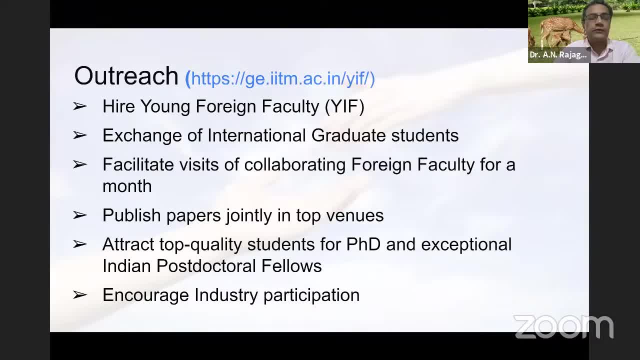 Then join papers in top venues, attract high quality students for PhD and also try to attract exceptional Indian PDFs And also, of course, in the process, encourage industry participation. And you know, along the way, we also want to. 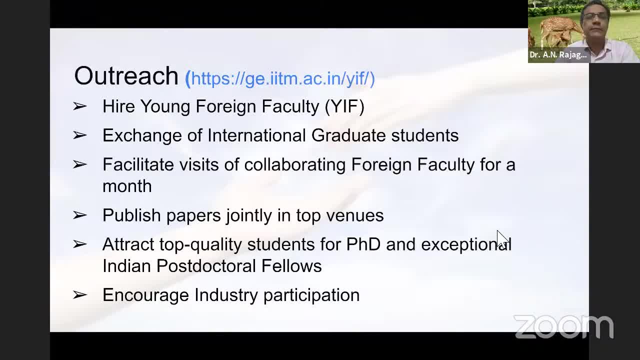 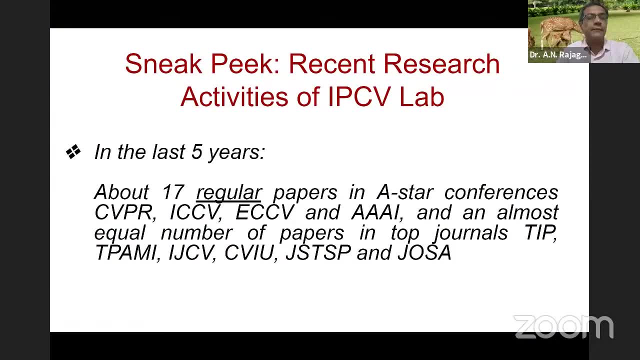 Yeah, Right And okay. So why? So? are we really up there? So, in a sense, I just wanted to give you, give you a sneak peek into all the recent research activities of the IPCV lab And I'm glad to share with you that in the last five years we have had about 17 regular papers in ASTAR conferences such as CVPR. 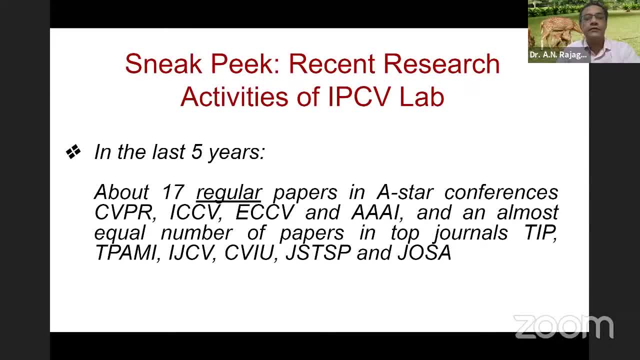 Those of you who work in vision would all be very familiar with these conferences: CVPR, ECCV, AAAI, ICCV and so on, And then almost an equal number of journal papers in TIP Time, EICV and so on. 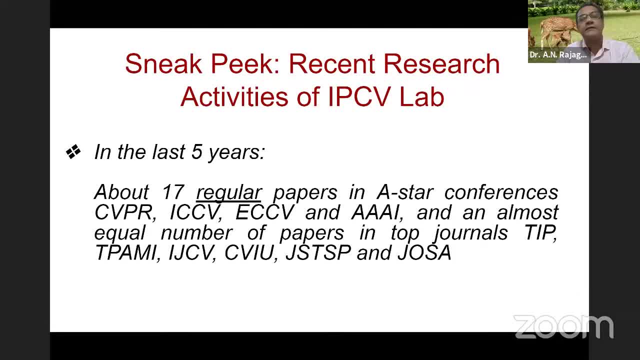 Right, So, So, So So, we are one of the most active research groups in the area of computer vision in India And and I thought right, And I thought I would spend spend a small amount of time trying to highlight some of the them and trying to talk about, kind of give you a glimpse. 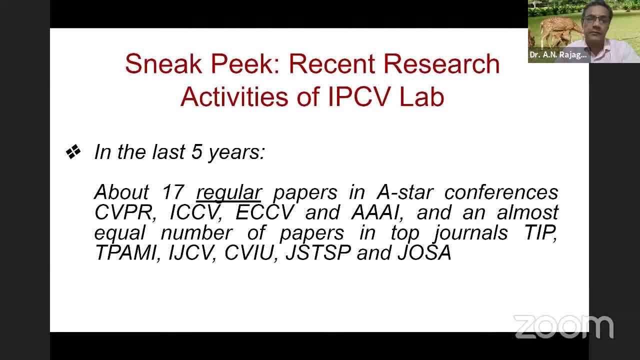 That's why I call it a sneak peek into some of the recent research activities that we've been doing in our lab. So I kind of set the tone And then, of course, then we will move on to things that we want to look, look ahead in terms of what we want to do as part of the center of excellence. 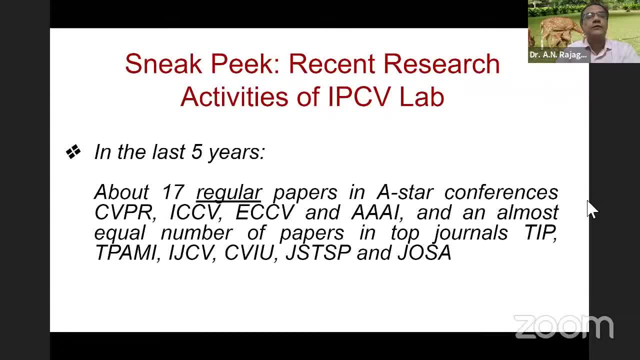 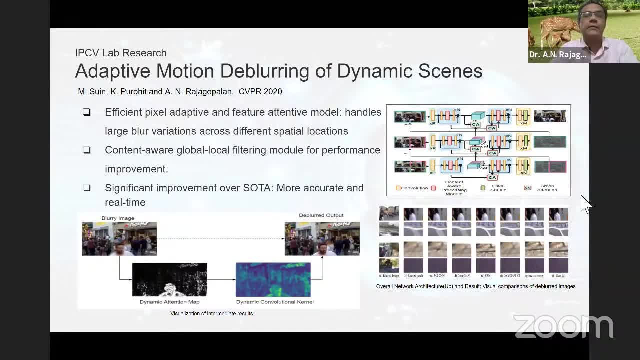 So let me kind of move on to the next one. So this is the first thing that I wanted to just introduce. It was about it was about the motion blurring problem. This is a CVPR regular paper, a 2020 paper. 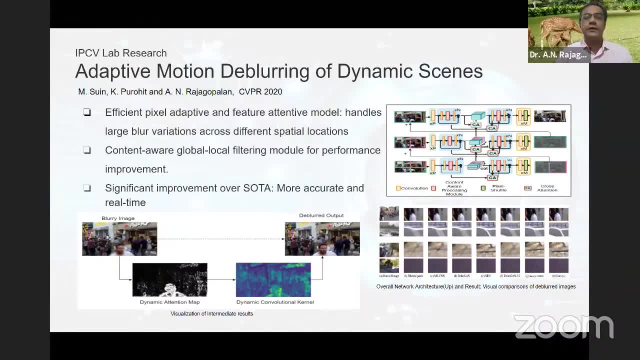 And here we have a motion blur until about a few years ago, And it was very important, I mean in order to see sharp images. people don't like to see images that are blurred. But then of late, it has gained even more importance because- because most of the deep networks are typically trained with deep networks- 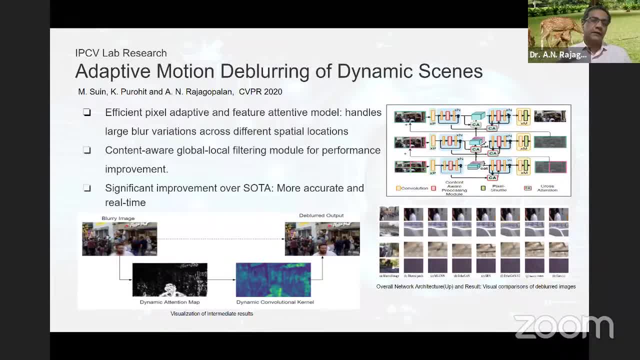 Right, They're typically trained with sharp images And therefore, when they, when they are shown blurred images, they can, they can kind of, they can- get stumped, And so that's the idea is to be able to be able to create sharp, sharp images. 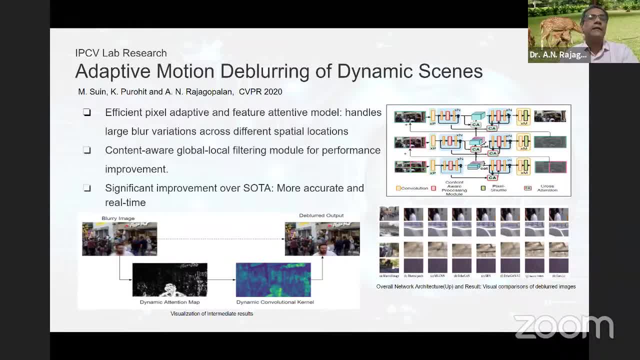 I know if you, if you kind of give a blurred image as a picture, And these are typically a hard problem, because what could happen is you can have a scene where you can have the camera that's moving. You can also have some objects that are moving inside the scene. 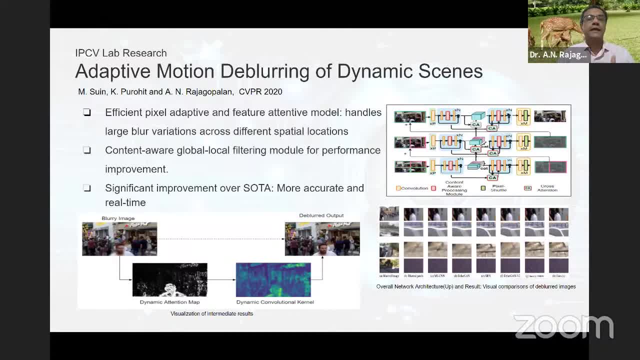 And on top of that, you can also have some sort of a 3D, sort of a depth variation, Which really means that you need an algorithm or you need a technique that is going to have all of these together. So, in this work, what we did was actually that. 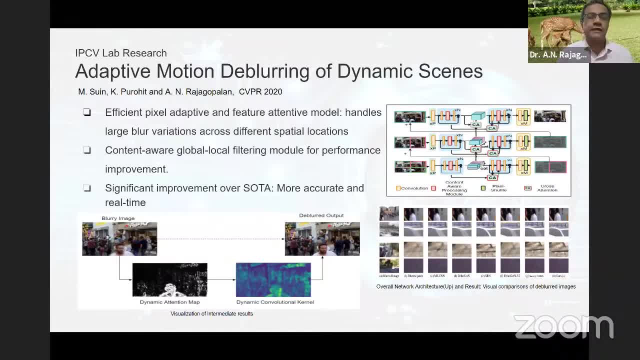 And what we did, was it brought in and sort of an attention mechanism, And we should also look at the global context as well as a local context through something called a cross of our attention and something called as a content of our attention, This kind of a patch, hierarchical kind of a framework. 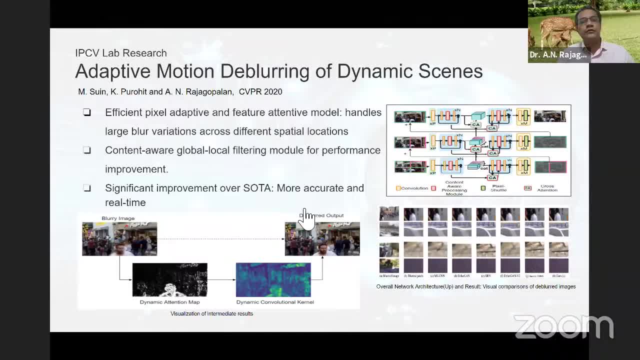 And, and of course you know, I have the details here For those of you who are interested. we can look at the details later when you have a Q&A session, If there is time, Anyway, I mean so these slides are going to be up there for all of you to see. 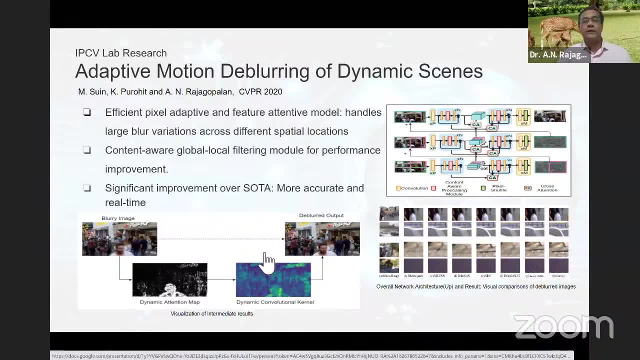 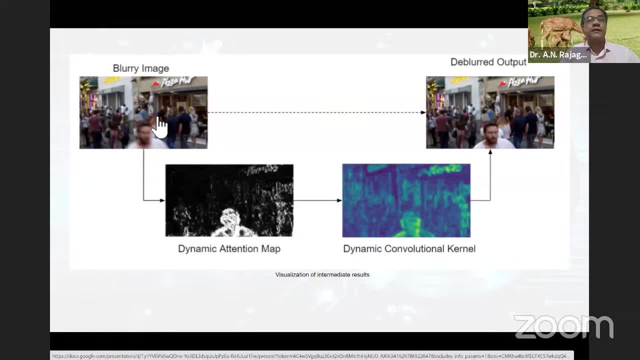 And then let me just share you one of the outputs that we have here. So, as you can see, on the left this is a blurred picture, And you can see that this guy in the front is quite blurred as opposed to others, And therefore what happens is we have a deep network that kind of tends to pay more attention to regions that are more blurred. 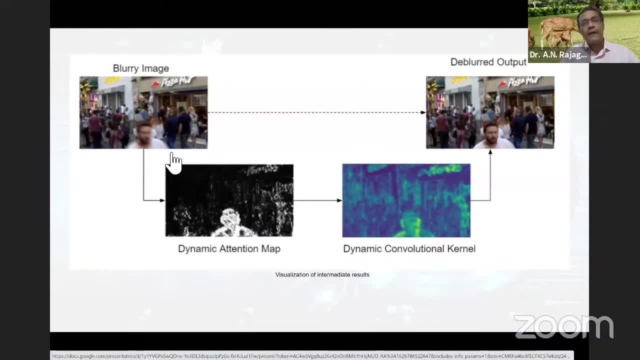 Which is what it ideally should be doing And so which is what it exactly does here. So, if you notice Right, So we have a deep network that tends to pay more attention on the person It was blurred And of course, it also pays attention to others that are that are relatively also blurred. 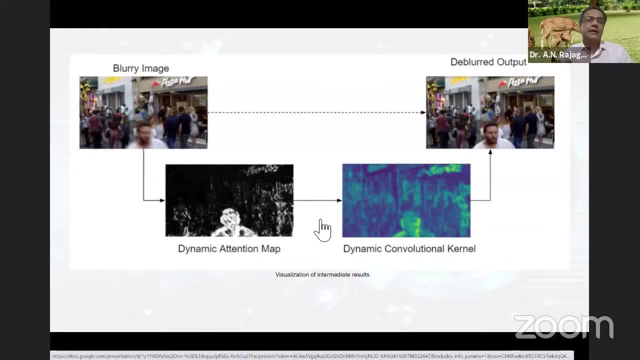 And then we also introduce a dynamic filtering colon, because, because we realize that it's not a great idea to have a colon that is no, no, that has a fixed set offset, So we introduced right into this deep learning sort of, into this deep network. 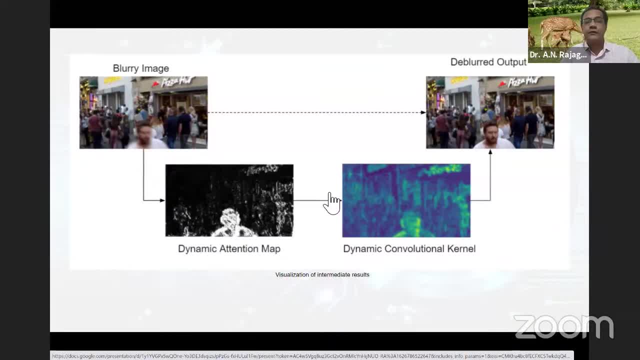 Also, you know, a facility to kind of to automatically adapt the offset of the colon, And which is what you see here, Which is about to start for the regions that are more blurred and then small for the other regions. Right And just you know. a quick look at some of these pictures, the show one: 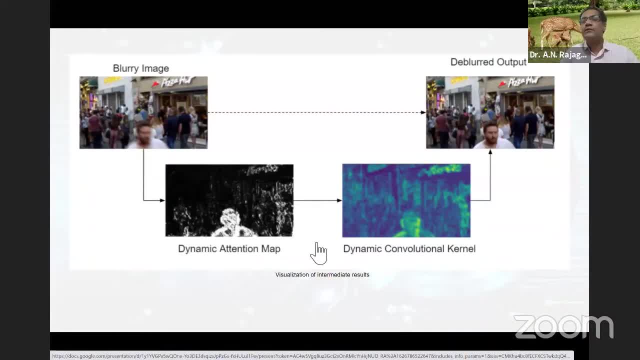 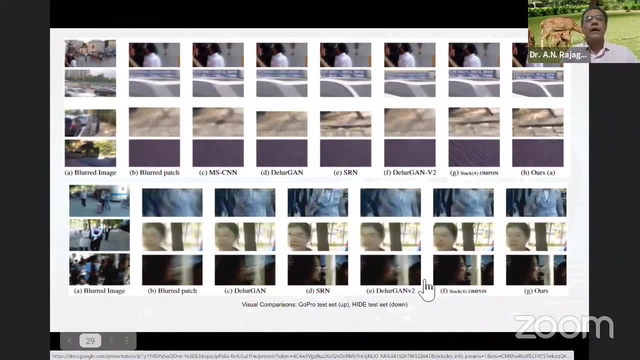 For example, if you notice this lady out here, you can see a picture coming out very clearly in our this one. It's kind of a state of the art to this method at that time. Now the our next one right which I want to talk about is is unconstrained motion: deep learning. 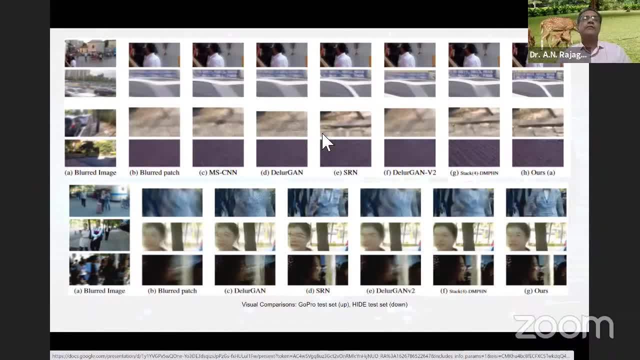 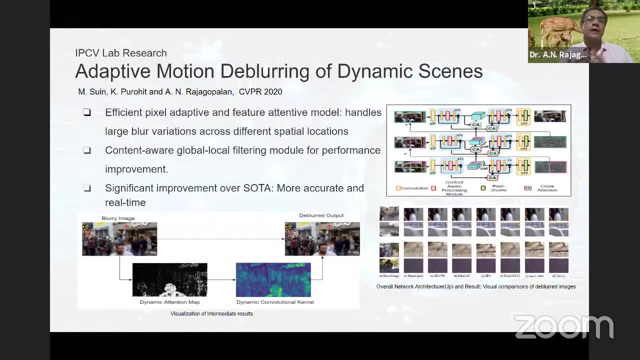 This is a traditional approach, This is a CVP or 18 paper. So here, Right, with multiple lenses, not just two, you can have three, four and so on. and therefore one kind of wonders: right, what does one do, right? uh, i mean, so one of the things is that if you had a blurred 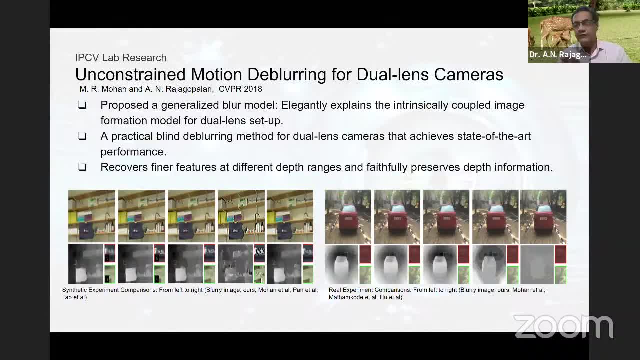 picture again. so the second talk is also about something you know which is related to motion de-blurring, and the idea is that you could take just one image and try some kind of a de-blurring, but then, but then right, given the fact that you have a depth dependent blur, you could actually 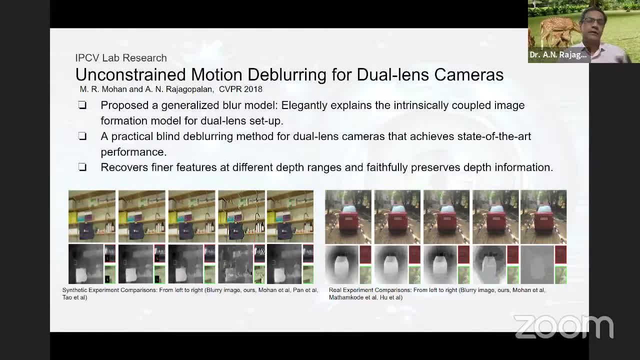 you know, you know, utilize the second image also, but you could have a blurred, because in this case you have a blurred pair. now, until our work, there were these other words that were trying attempting something similar, but they used a constrained sort of a setting which meant that these two cameras 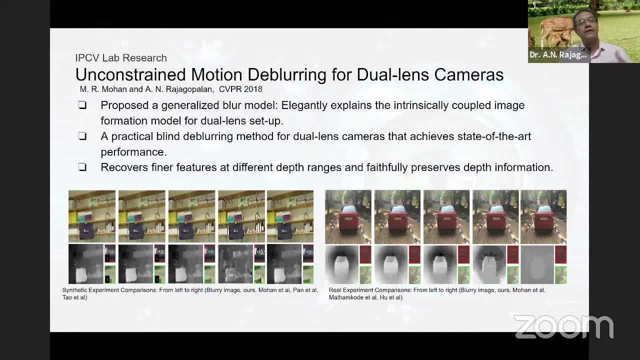 would have to be identical. so we kind of relaxed that we said that one of the cameras so you could have a wide field of view, narrow field of view, you could have different exposure times, you could have a resolution right which may not be the same in both the lenses and yet right you would want to. 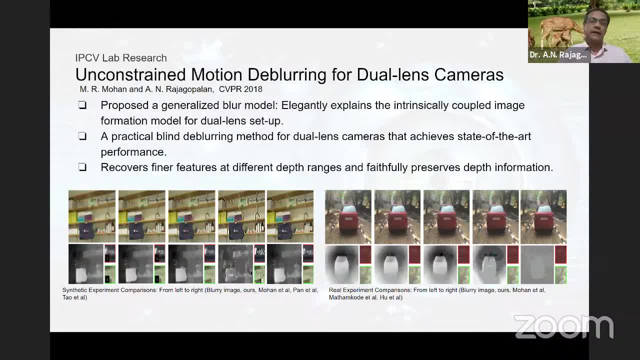 do a depth estimation, come and come, sort of sort of a deep learning right, and we actually showed that this is a fairly ill-posed problem. it turns out that if you try to estimate the motion density function for you know, for, let's say, each of the cameras or each of the images, then what can happen. 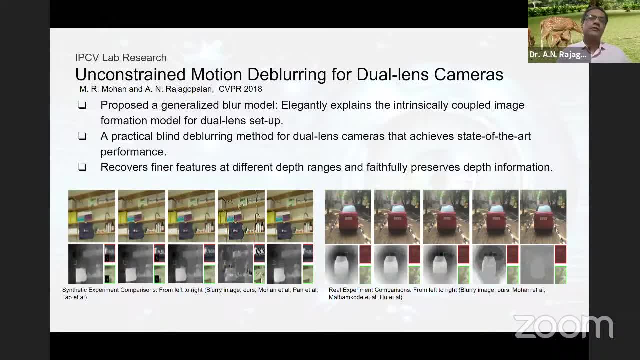 is you could have a drift, right, they could. so both mdfs could have a mutual drift which can actually give you the observed images that you're actually seeing. but then you know, it can lead to a left right inconsistency in terms of the stereo cue right. so we actually solved this problem and we 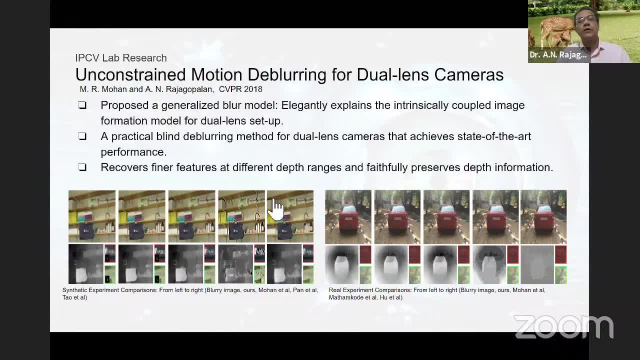 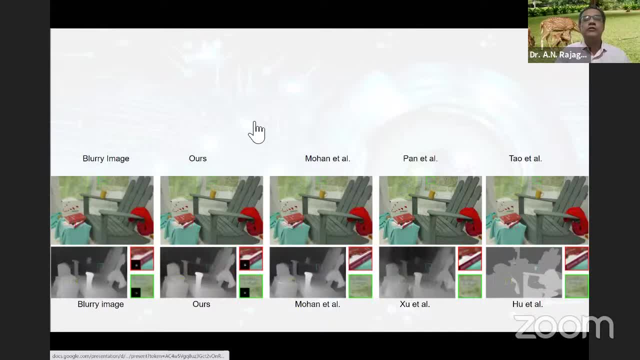 showed that you know in the process. i mean, you could not only estimate depth, but then you could also create sharp pictures. and instead of going through everything, i would just ask you to ask you to look at these small, zoomed in sort of sub images, right where you get an idea about you know what kind of, what kind of- uh, what kind of sharpness we. 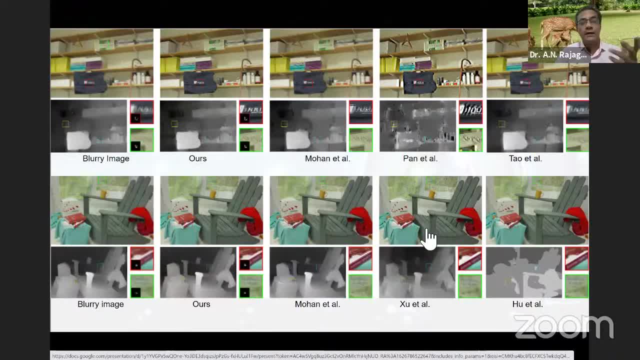 get, as opposed to other methods, which struggle typically right when you have cameras that are anything straight moving on. uh, the next one right which i want to talk about is actually bringing blurred- uh, bringing like blurred moments. now, this is a cvpr 2019 paper. this is the first time in 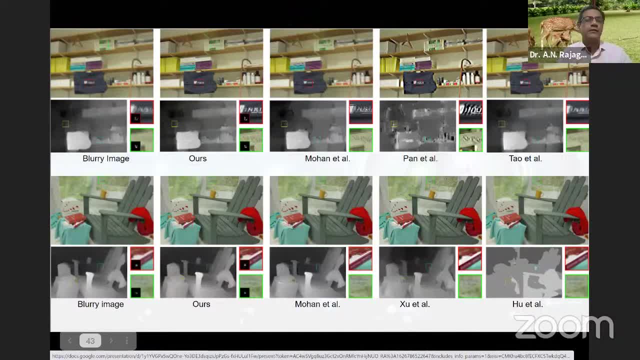 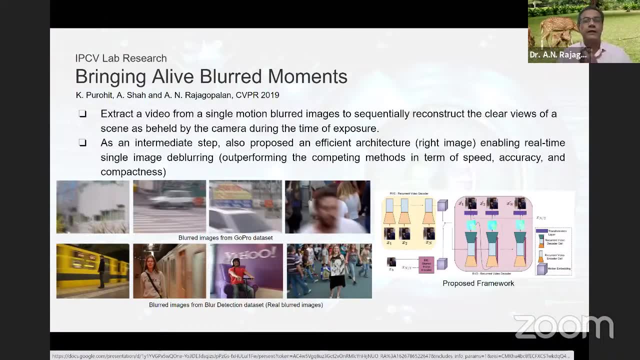 fact, ever and until this work right, people were always talking about creating a sharp picture, given a blurred picture, and then we, for the first time, i talked about how actually one looks at how the camera is moving and what happens is, you know, you have a camera in action. that is kind of you. 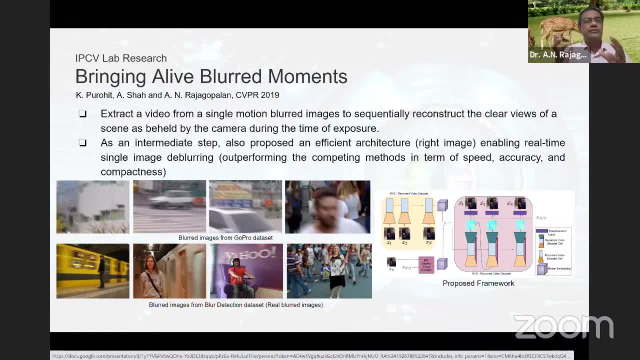 know, that is kind of witnessing the scene, and during the exposure time a lot could happen. your camera could be moving, you could have dynamic objects right, which are actually moving in the scene. you could have depth differences, right. people standing in the front, people standing somewhere else behind, and all of that and all these, what versions right? in a sense, then you 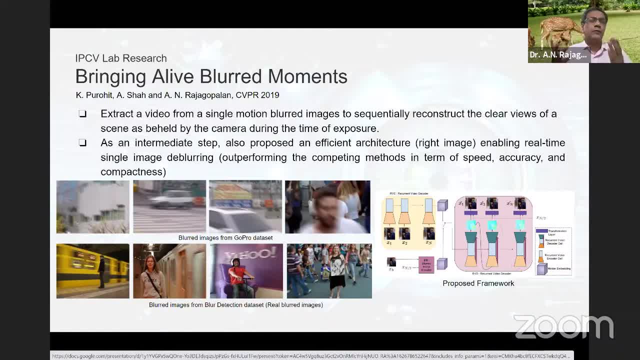 have a weighted walk of all these, or a weighted walk of the latent sort of a sharp image right, which you would like to ideally see, and what happens is you have this average of all of this and you know, when the shutter snaps, right at the time, all that you get is one sort of a blurred. 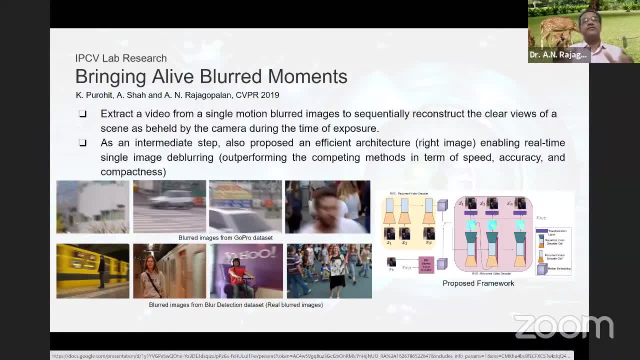 picture. so because, look at, the blurred picture looks very dull. of course you can sharpen it, but then we went one step ahead and we asked: we can get a real, real of what exactly happened during the time that the shutter was on. so i'm going to show this show, this video, right where you can see. 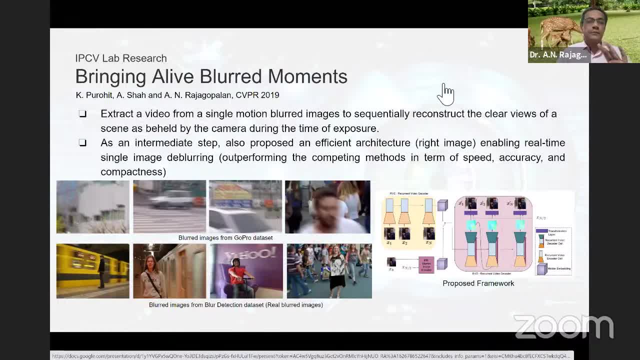 that the first images, the first row is all still. you know, images. these are all blurred, but then out of the blurred image you could actually create a video and, for example, the last was other output. so what really happened during the time that the exposure was open? right? so obviously this was. 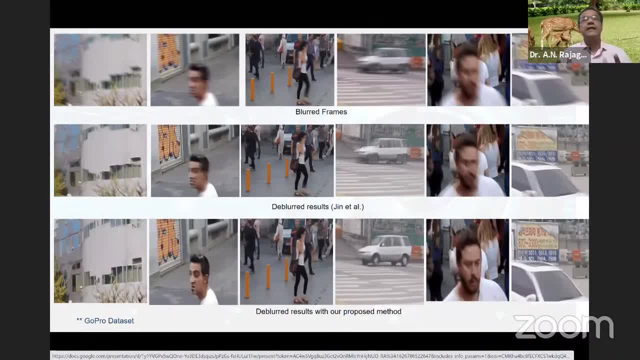 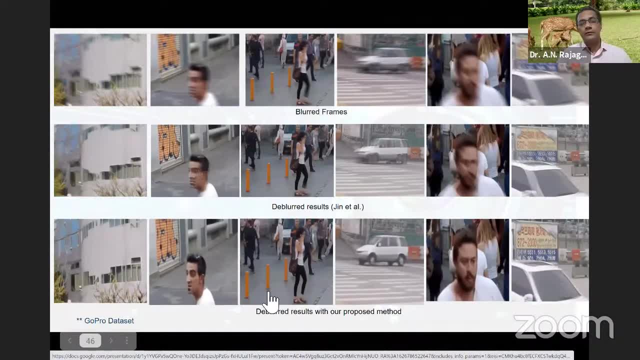 the very first work, right of its kind, to actually tell that you know, you could actually produce a video from from a single sort of a blurred image, and i would also like you to, you know, to kind of take a look at this lady's leg, for example. it's a very, very local motion, right. you can see that. 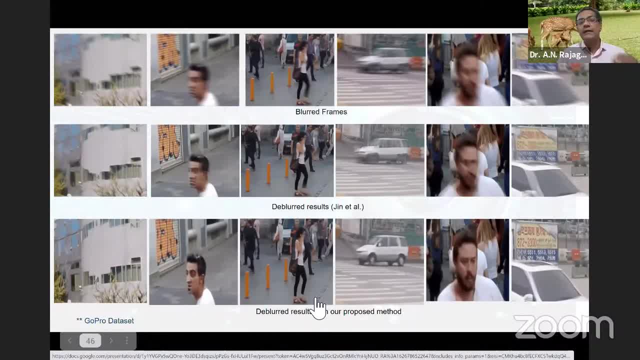 she's shaking her leg and and you know even something like that right, you can actually locally capture. so not only captures global camera motion, it also accounts for any local sort of a sort of emotion right which can happen, and it kind of relives, right what you might like to see in a kind of a blurred image, right, so kind. 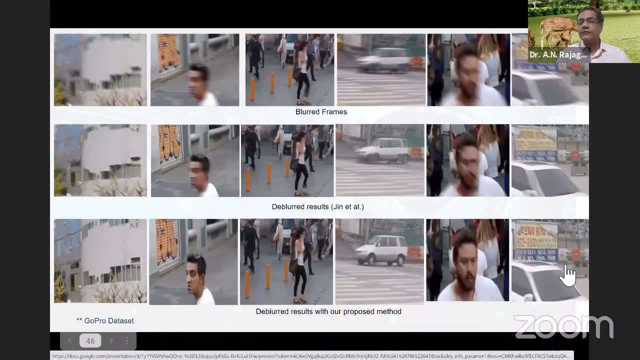 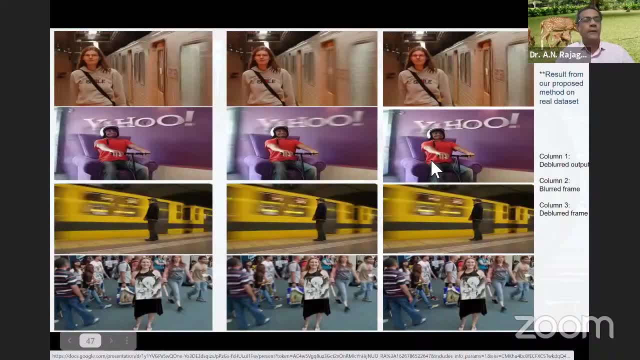 of very, very first work up in skype, uh, and of course there's, of course you know, one more, one more case. okay, let me go and now the next one right that i wanted to talk about was kind of unrolling the shutter. so we all know that. you know, most of the cmos cameras these days come with the 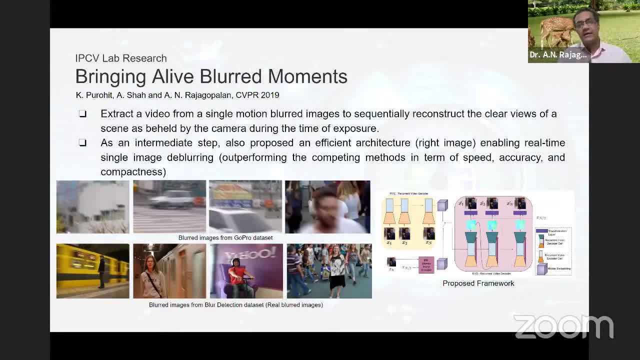 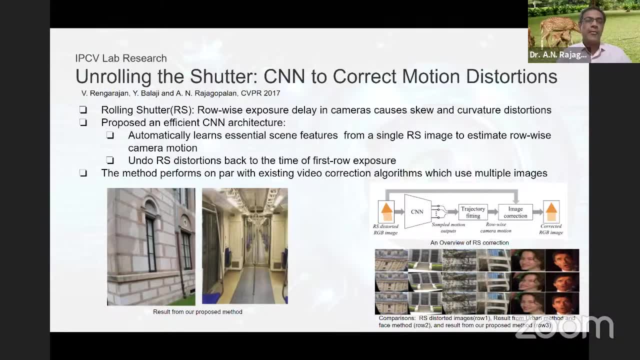 rolling shutter, which means that not all rows of the sensors are exposed to the same camera motion right. so what the first row sees is probably not the same as what the what the last row sees in terms of the camera motion right, and- and this really matters- when the camera motion is fast enough or if there is an object right which is moving, that is moving. 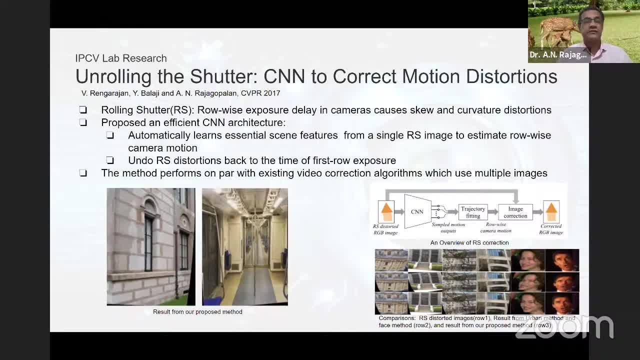 fast enough, right, you know, as opposed to the supposedly shutter time and so on. so so here, right, what we actually did was. so one of the things that you really need is in order to be able to able to rectify, and we know that if there is camera motion, then our general notion is that lines will 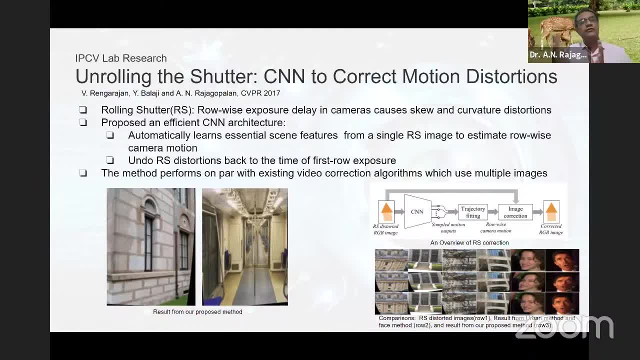 remain lines, and if there is, if there is an exposure that is too long, you can at most get a blurred line, but then a line right will stay as a light. but then what happens is, in case of a rolling shutter, when there's camera motion, the light can bend right, like for example in this: 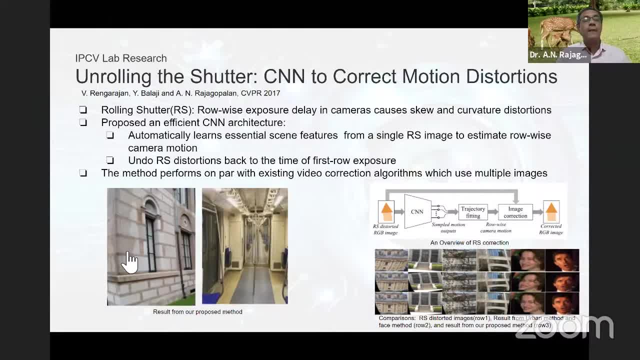 case this building that you see. here you can see a bend right happening, which is actually not true. the original scene doesn't have the bend, but then because of the camera motion, you can end up seeing a bent sort of a. you can see bent lines and so on, and therefore this work actually takes that into. 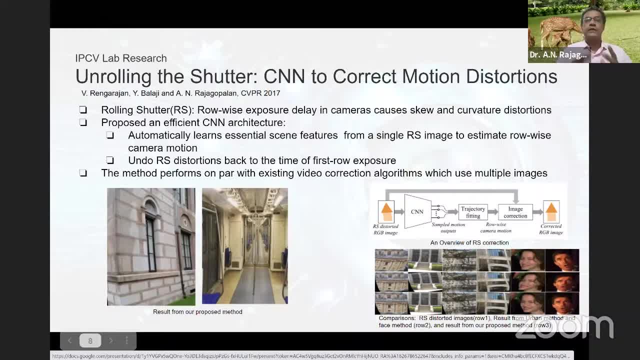 account and it is a kind of a parametric formulation within a deep network, and what we typically solve for is really an x translational motion and then a rotation along, along the z-axis, and we solve for this, and then, of course, and what you really need to do is estimate camera motion for every row. 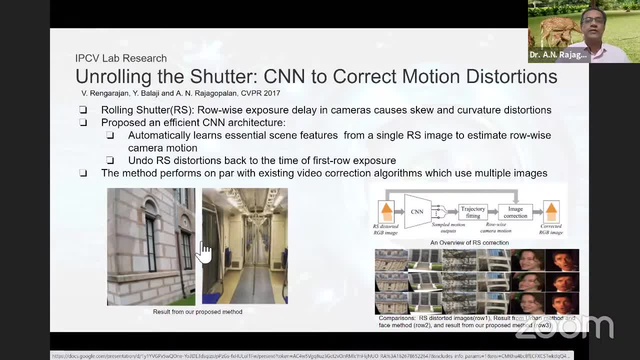 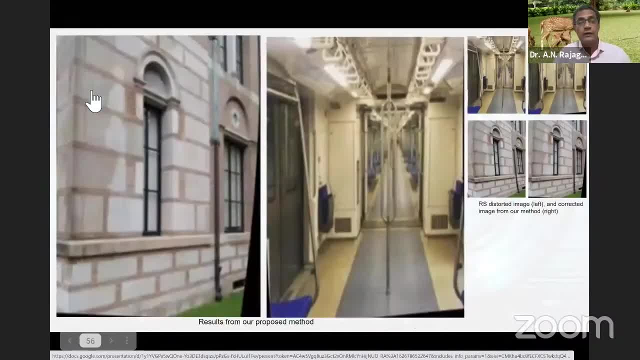 of the building so you can see the camera motion interpolated and then you can actually unwalk in order to be able to see a rectified image right. so i'm going to show this blown up picture so you can see that after rectification these lines become: the building looks looks vertical, otherwise it. 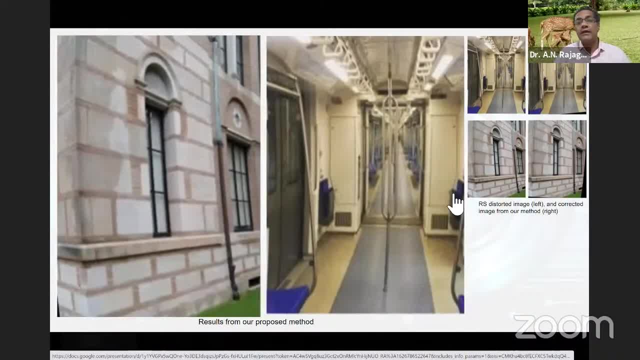 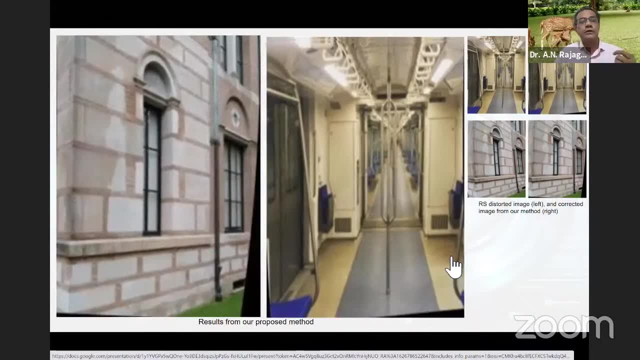 looks like. you know, one of the wall is the wall edge is curved. similarly, this is inside a train, right, you can see that. you know the. the bent is removed and uh, and of course, here are some still images. the nice thing about this work was it could do it with just one image, well, during that time. 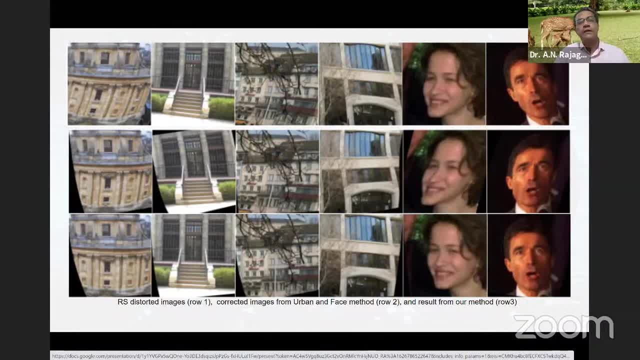 the state of the art was that you know you needed multiple images in order to be able to do it, be done with just a single image. here is a skill image, for example, for a certain class like the face class. if there's a rolling channel effect, you can see that. you know there's a skew in the face. 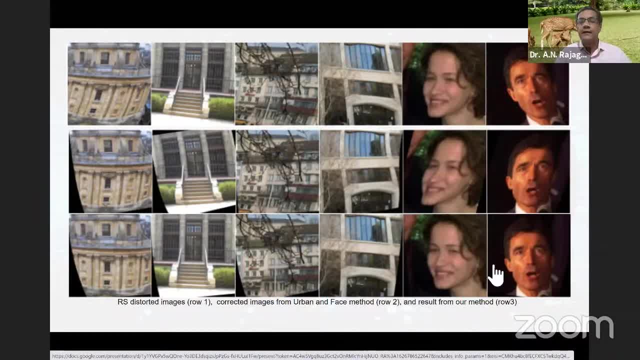 but as well as after we run our, our other submitter. now you get the faces as you should normally be able to see them right, going, moving forward. let, uh, we also did. we've also done some works on robust super resolution, and especially for the unpaired case, because that is what is most challenging. 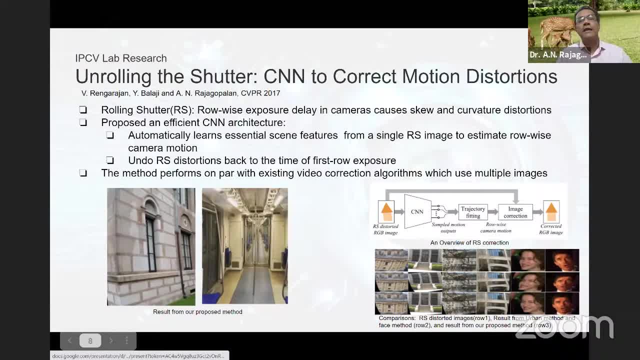 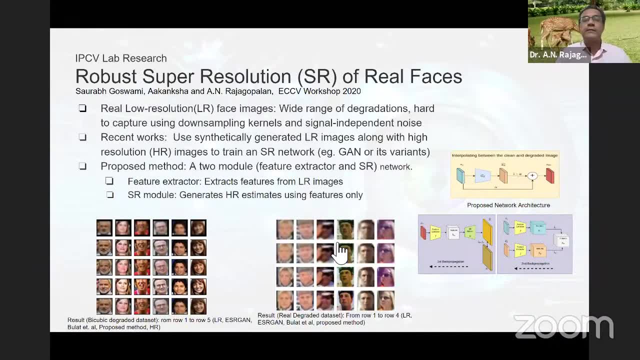 and, and you know, these days people are looking at problems of the kind where, let's say, you have a really very severe you know, not the kind of things that we're seeing like five years ago and, for example, you know we did some work, you know where we showed that, even if you had a picture- 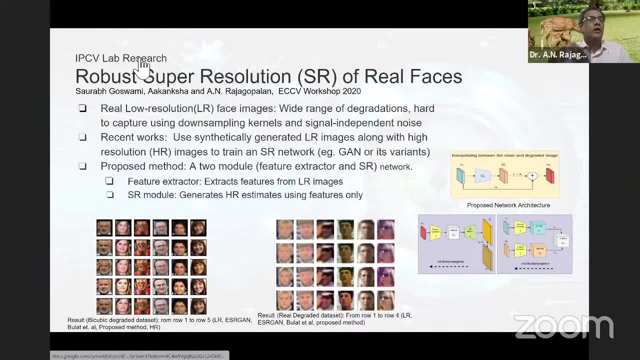 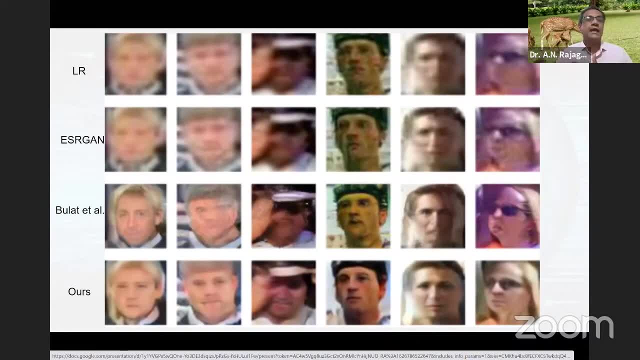 which is as bad as this, and there is no paired version for this. you don't know how the, how the high quality image of this guy looks like, but it's called the wilder phase data set and uh. and then you know you can't train with with a pair, where you, where you know the person right. so this is. 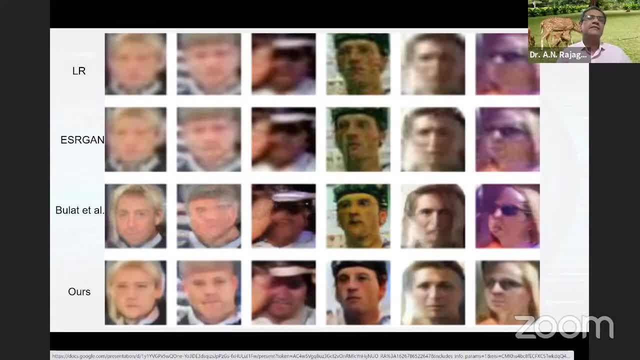 kind of hallucinating, but but then hallucinating, you know, in a sense, that you know which kind of which you know sort of emulates what, what we as human beings are able to do with this kind of image. so what we as humans do, so what we as humans do, is that if you have two pictures- low resolution, 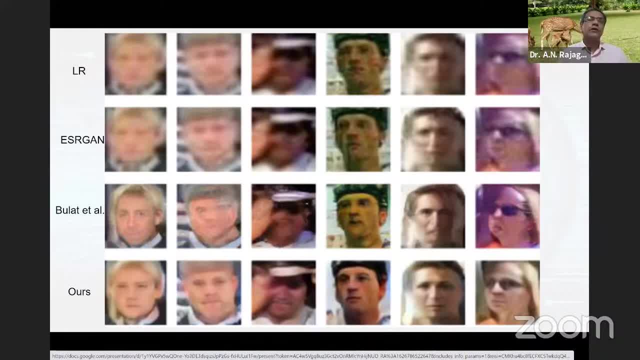 of the same person. but then if they're going to see degraded, you still want to sort of say that you know it's the same person. so this kind of a deep network does exactly that and you can see here the output. so you have a low resolution picture of this guy and then of course it's 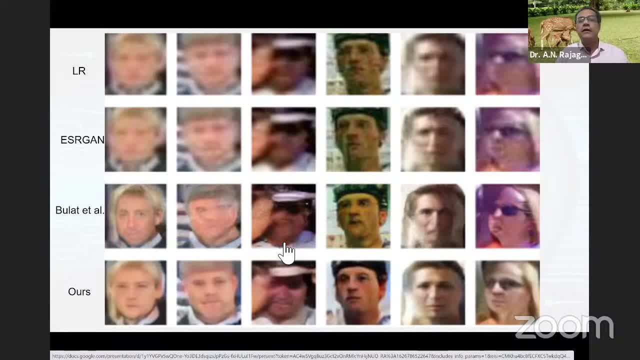 very hard to really prove whether this is correct or not. but then you know it can only be sort of right, a qualitative sort of a judgment right here, where you kind of see, and then you look at the picture and you sort of believe that yes, right, i mean it's doing okay, right. and then the next one: 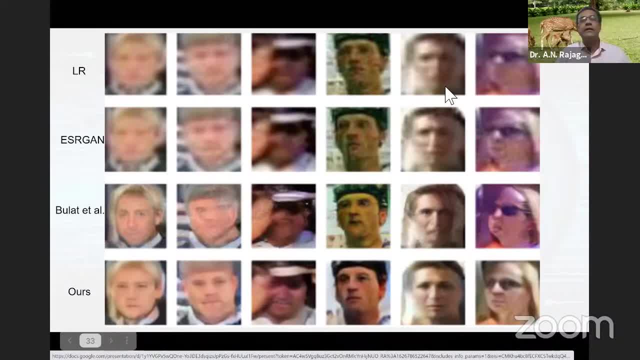 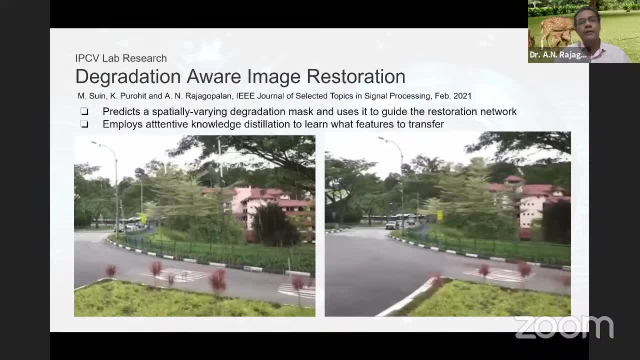 is a degradation of that image restoration. there's a reason paper in uh, in a, in a special issue of jsdsp in february 2021, and here it is about, you know, a deraining problem, and there's not just for deraining. this can be even applied for raindrops or if you have whatever. i don't. 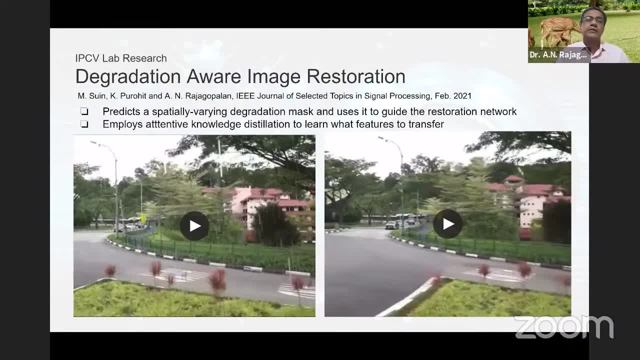 know anything that is spatially varying, and if you had a degradation that was spatially meeting, waiting, right and uh. so in this paper, what we actually proposed was you know, estimating or learning- uh, learning a degradation mask that is spatially varying, and then use this mask to 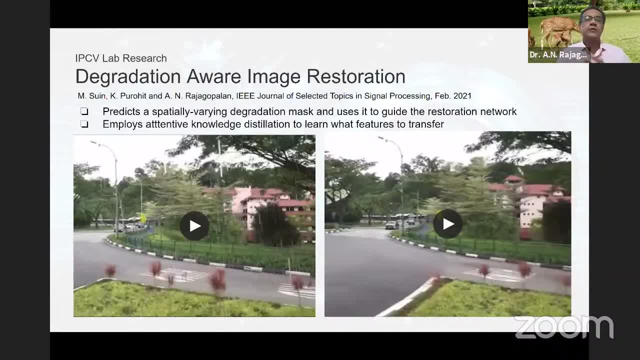 kind of guide the reconstruction process and uh right, and this mask also tells the kind of reconstruction network where to focus on. for example, when we say this, when we say that this degradation is spatially varying, what we really mean is: you know, there are, there are parts of this. 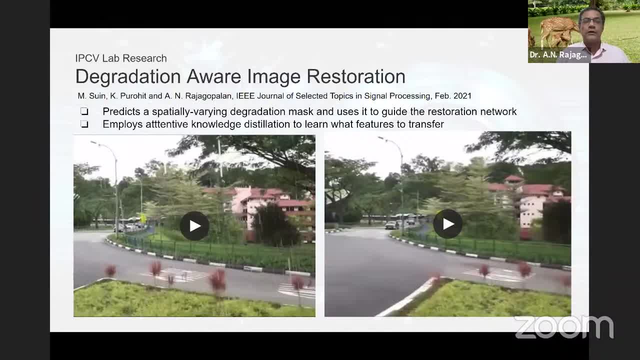 scene which are totally unaffected or very little, or, or which are seldom affected or very little affected, and there are regions which are which are affected a lot. for example, i'm going to play this video where, on the left, you'll see a rainy sort of sort of a scene and on the right, when you see 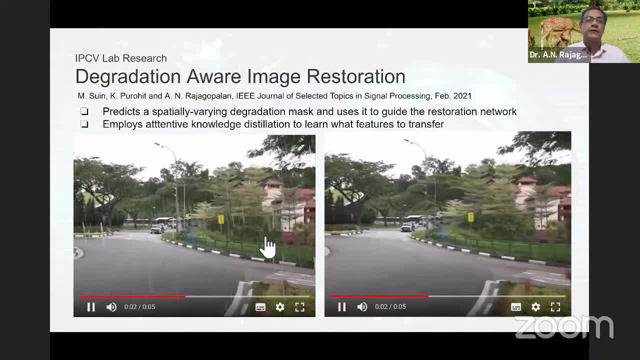 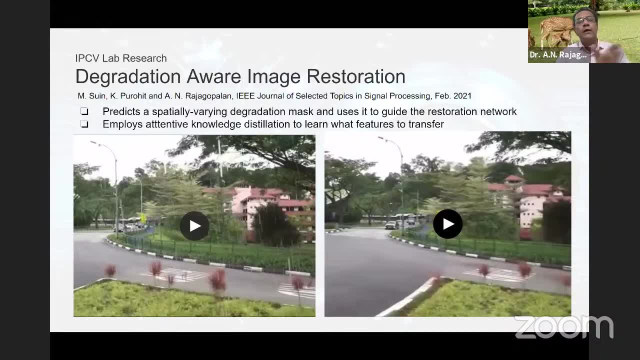 the rain and you can see this is a very small area and there's a lot of dead rain and it's not a big thing and you can see it's very low right, and this is what we mean by the space in the lighting- sort of sort of degradation. moving on, uh, the next one that we did was again that these 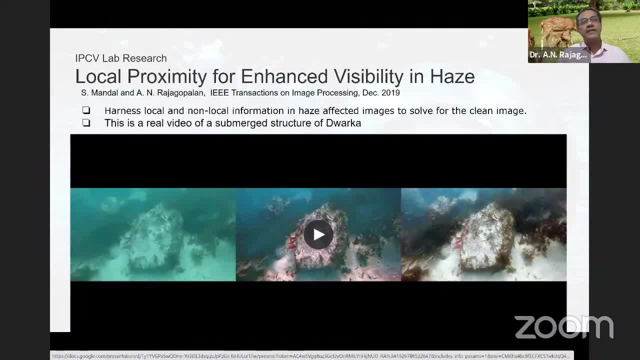 are all unpaired. you know, in all these cases you won't have. some of them are clean event, for example. you don't have a database. well, as you know, somebody took a scene on a day when it was very, very nice- no rains and nothing- and then, from the same viewpoint that the same person took another. 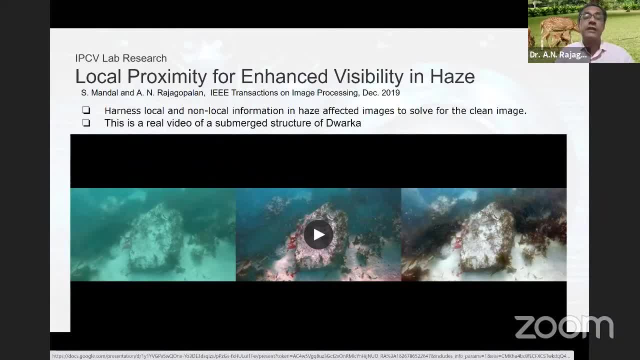 picture right when it was great. it's impossible to have situations like that, more so if you're looking And underwater. it's especially impossible to get a kind of a pair where you have a clean image and then you have a pair for that which is actually a degraded version. 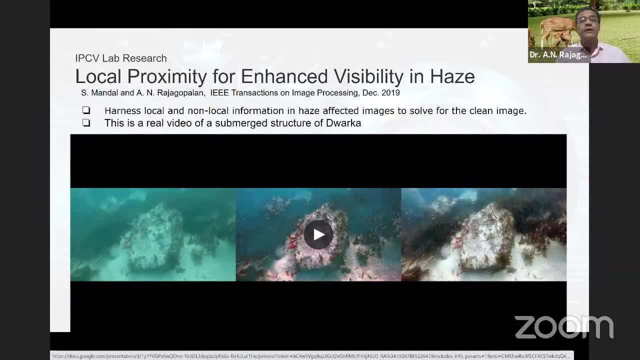 All that you have are hazy images. Now, the one that I'm showing you is actually at Dwarka. This is from this one, This place, Dwarka, which is actually a city in India. Part of it is actually submerged in the water. 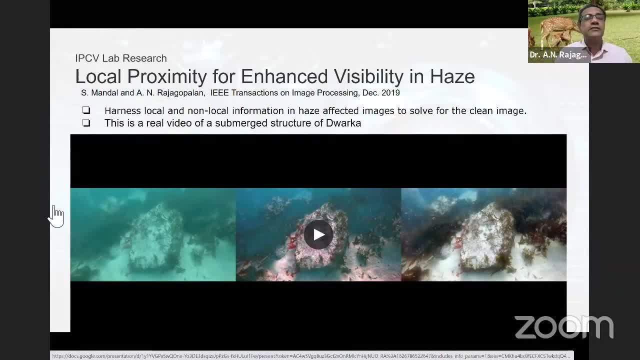 This is the banks of the Gomti River, And this is a video that was shared with us by the NOI-O people, and they wanted to see if we could actually restore it. So this is a TIP paper of 2019, where we used the idea of local proximity. 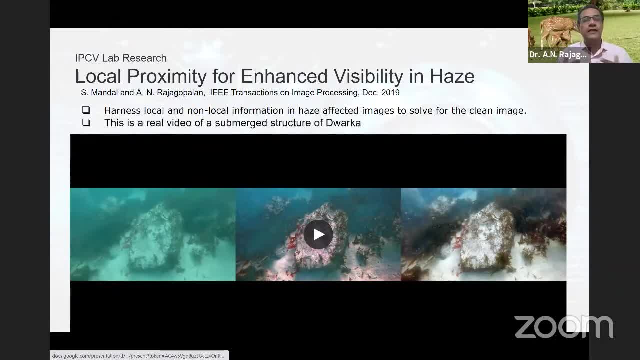 which basically means that the attenuation and the air light are the two important factors which are going to contribute to haze. So we kind of assumed that to be locally constant, and then we used non-local means in order to be able to estimate the irradiance. 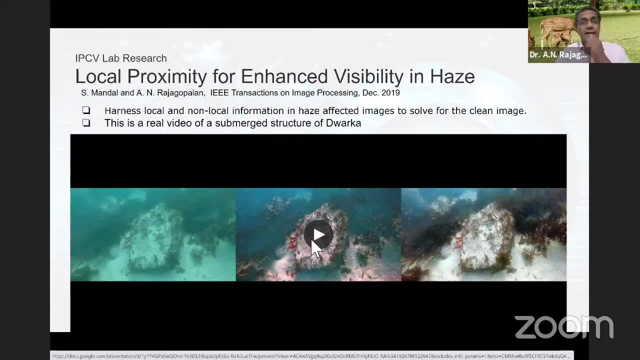 By doing that, we actually showed this. So after doing that, we can see clearly that, of course, in this we don't have a groundwater, We don't have a ground truth at all. right, There's no clean, unclean pair or anything. 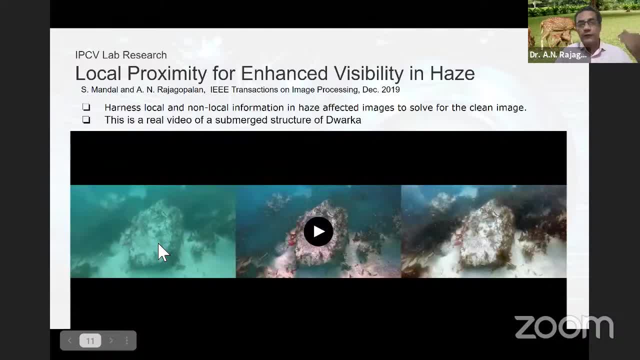 All that you have is a kind of a hazy picture of an underwater scene. The one that you see on the right is a reason method that is deep learning based, and the one in the middle is our method. So our seems to be doing reasonably well as compared to a deep learning method. 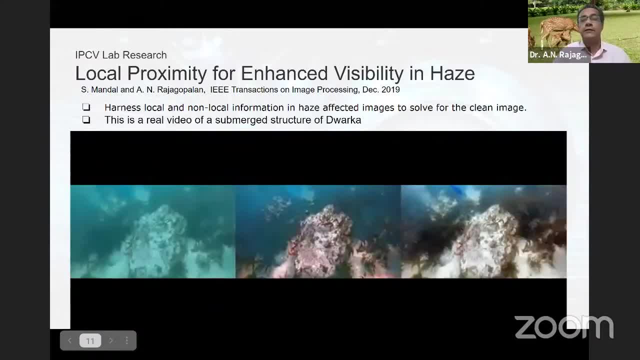 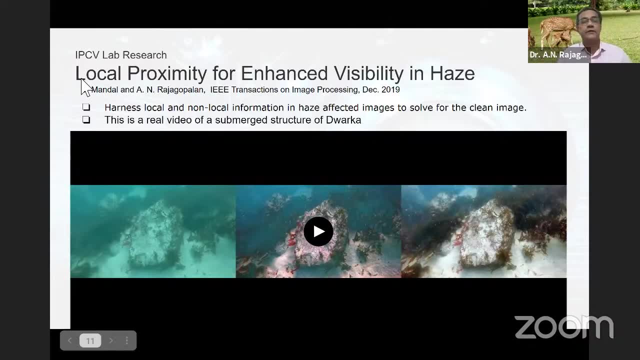 that has probably been learned to several hundreds and hundreds of images. Let me now move on to kind of going forward. What activities have we planned for the center Right now? we have kind of identified three main areas in which we think are very exciting as we go forward. 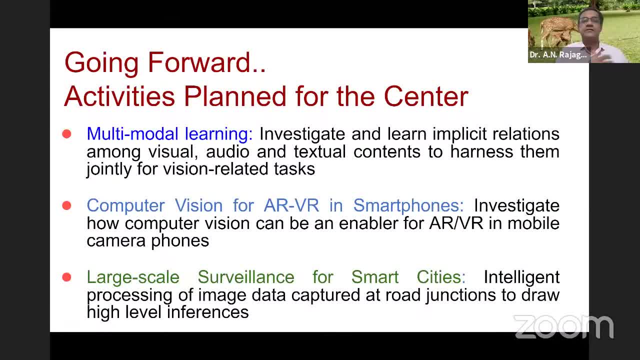 and you will see that these are not just an incremental version of what we are already doing. What we are doing- I showed you some of those things- And going forward, there's a major kind of shift in what we want to do. So we want to do something like multimodal learning. 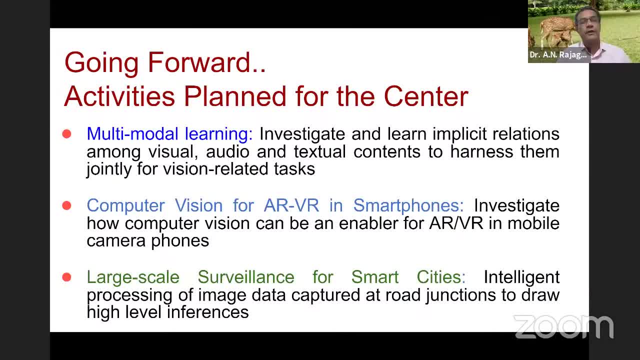 Now that we know that the web is flooded with all kinds of data- visual, audio, text, language, all of that- So we want to kind of learn the semantic relation. It's kind of loose, There's no kind of tights. 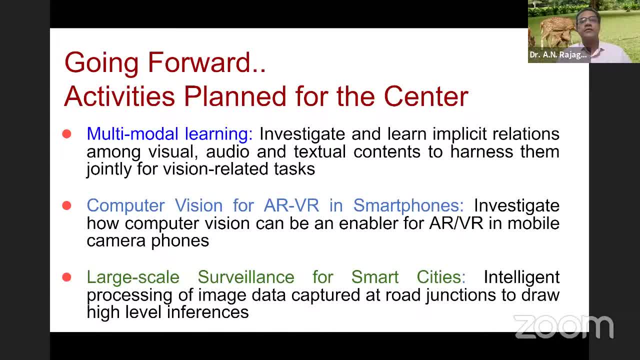 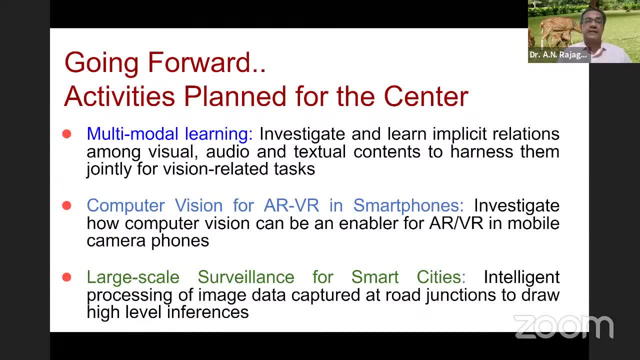 We want to harness them in order to be able to solve some of the joint tasks right. And the second one that we are looking at is computer vision for AR, VR and smartphones, especially for smartphones, you know, which are kind of handled and so on. 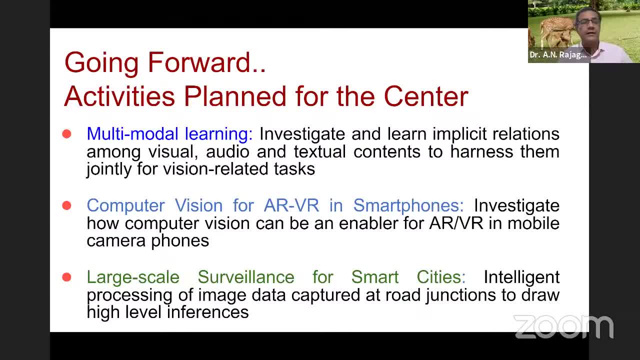 not for the general AR VR right, That, let's say, everybody probably knows that a lot of people are doing. And then we are also interested in some kind of large-scale surveillance. but large-scale surveillance, you know, just from the point of view of road traffic or road traffic. 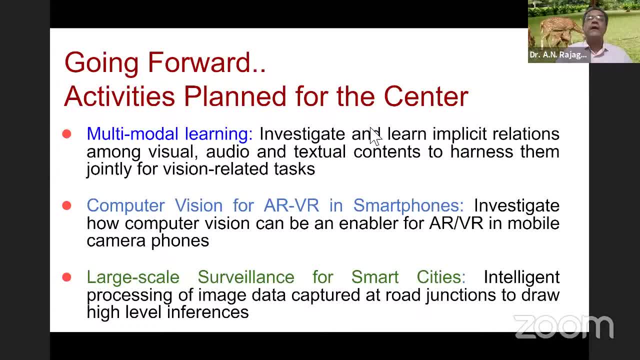 management and so on. I mean not in its entire sort of generality. Then okay, now going forward. okay now just to kind of motivate, right, what I mean by multimodal, right, I'm going to play this audio first, and you know, and kind of, if you hear this audio, 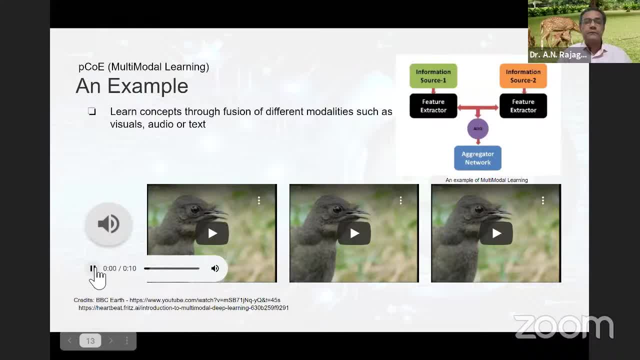 I hope you are able to hear Professor Choleba. are you able to hear the audio? Yeah, yeah, I do, I do. Thank you, thanks, Okay. so now when you hear the audio, you know that they're not birds, right? 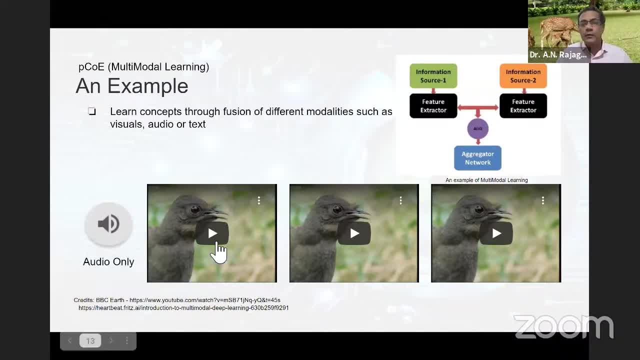 They're a bird, but then, beyond that right, you don't have any idea about, probably, what's happening. Now I'm going to play this video right Here. all that you see is a bird right that's walking around. 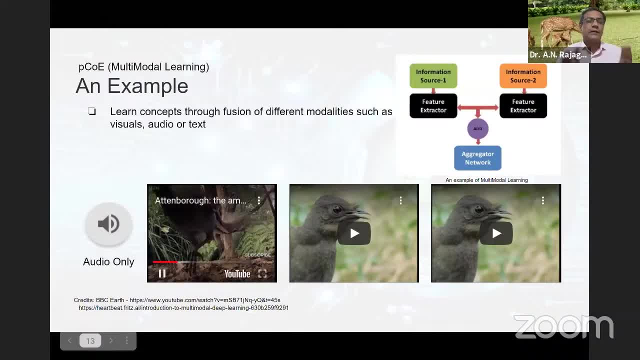 And then all that you have is that information and maybe right it's doing something. Now, if I combine both right, if I give you a picture like this where you have the same audio right which I played you before, 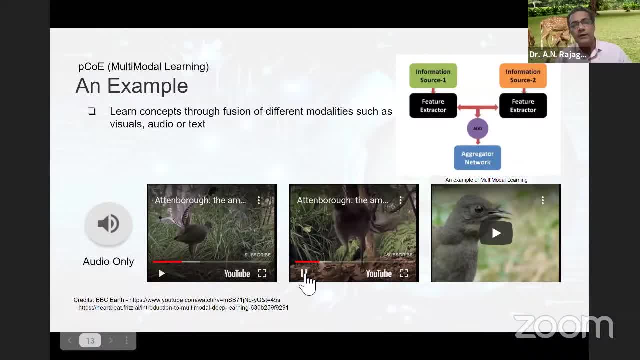 and now you have a lot more information, right, You know that. okay, there's a bird, and there's a bird right which is also making this noise. And going one step further. right, I'm going to play the next video where you'll hear something. 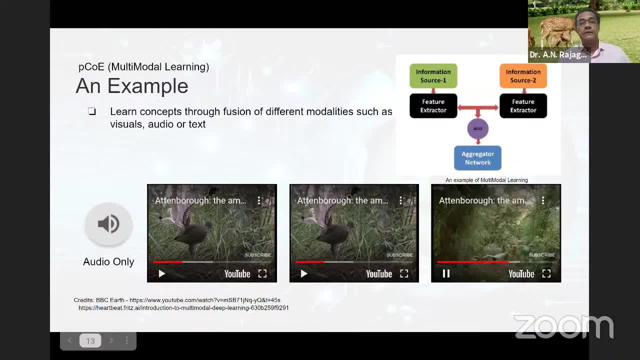 He also, in his attempt to out-sing his rivals, incorporates other sounds that he hears in the forest. That was a camera shutter, Right, Okay, so you kind of heard that right. So what this means is that I mean right with, let's say, video alone. 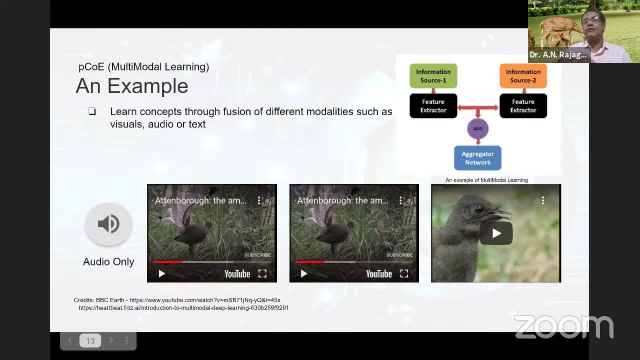 with video plus audio plus video plus audio plus some language plus some text- right. all of this boosts our ability to know what is happening around us, right, And which is exactly okay. what we want to do Now. when I go forward, one of the first things that I want to talk about is vision. 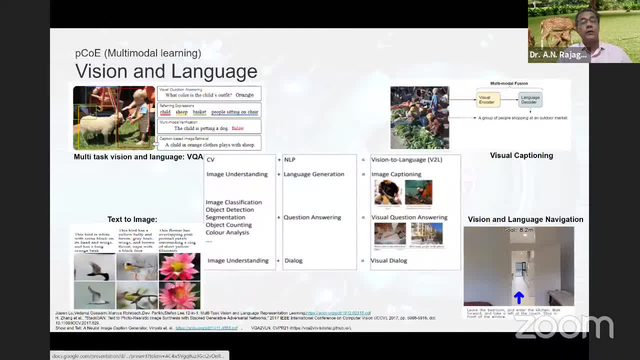 and kind of language, how these two can be married together. And there are already works, and from now on, whatever I'm going to be talking about are all works that have been done by other groups- right? Some of our works are under review. 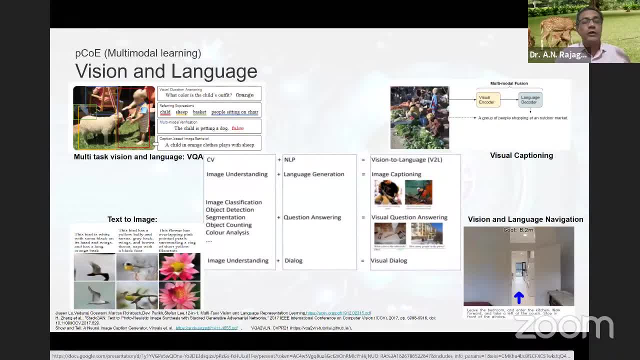 The ones that I'm sharing here are the ones that are already out there, And if you want to know who has done it and so on, there are these links below Right which you can click on if you want to read any of those papers. 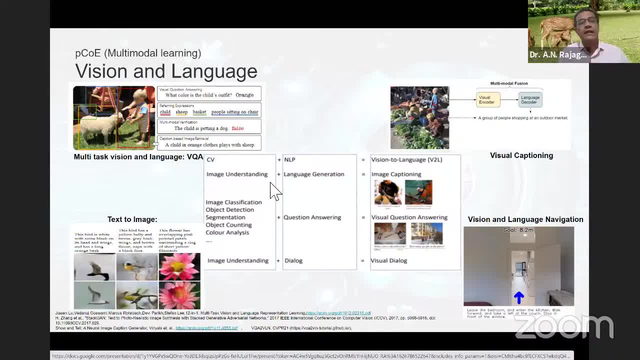 Now, just to start with right, this is a caption. So when you have vision and language, I mean you can have so many of these research problems right which actually revolve around them. One of the first right which I thought I'd share with you is about the captioning problem. 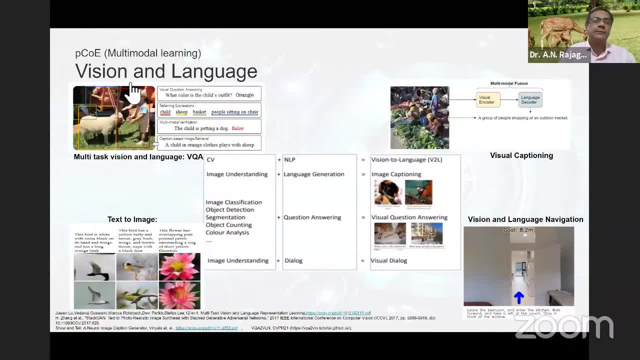 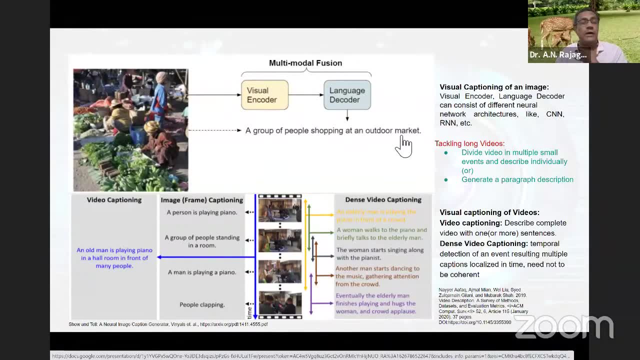 So in the captioning problem what you have is you know you show an image to a kind of deep network and then you want it to summarize what's happening right in the image, For example, in this case you show this image and then you expect a caption like that to come up. 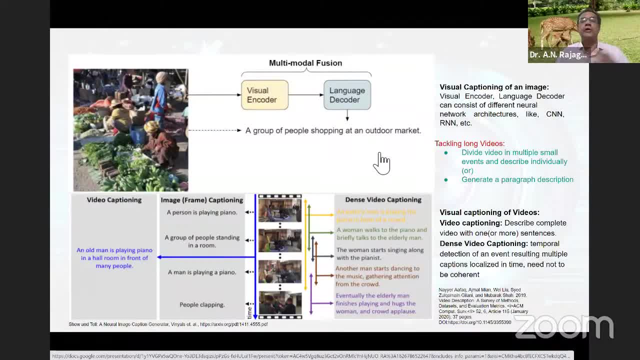 Right In this case. here, that's, you know whatever a group of people shopping at an outdoor market, right, which is what you want this kind of you know deep network to do. And the way right this is kind of typically done is you have a decoder. you know which is an RNN. 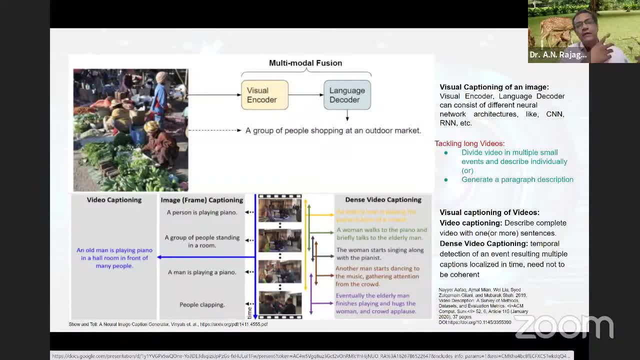 typically an LSTM, and then you have an image from where the visual features right you get. This could be typically a BGT network or an RSNet or something, And then these go as encoded features and then these go as input to a decoder. 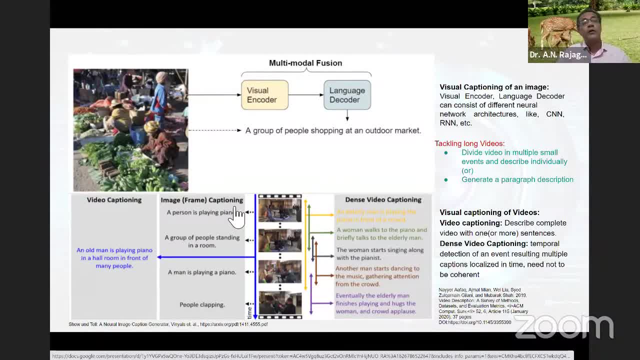 which is your LSTM, and then right, have in outcomes this sentence. You can actually go for that and then do. maybe if you had a video captioning you can do a frame-by-frame captioning, but then three by three captioning will lose out on the temporal connectivity. 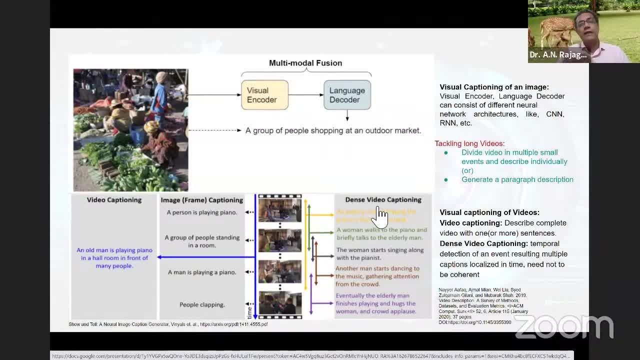 But if you do a, do a dense video caption, that's when we can get different captions and then you can actually associate one caption to another Right. So these are the already works in this, including some from our own, some from my own lab. 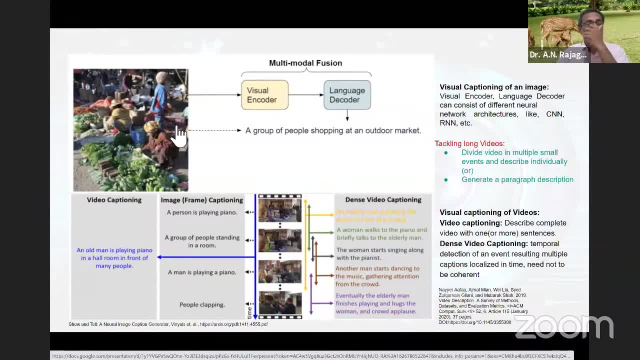 Let me just go back and then the right to talk about that. I talked about another problem which is even more rich in the sense that you know you can start asking things, which is called BQA, the question answering. So here, what you could do is you could show an image. 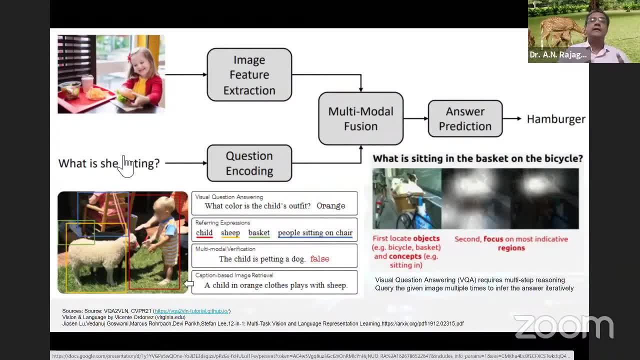 and then somebody could ask: right, So in this case, what is she eating? And again the output. I mean you want to say that no, no, no, she's eating a hamburger. And the idea here is that right. 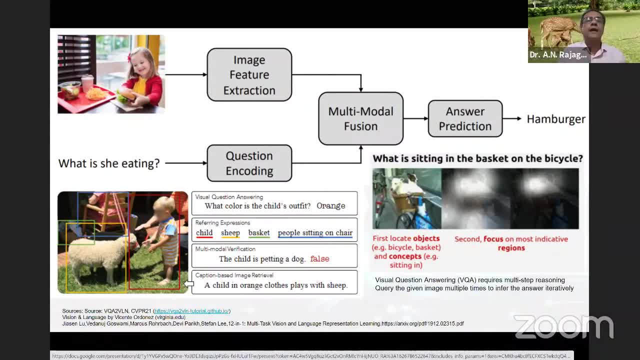 I mean you have sort of a, so you have a text embedding, and then you have an image feature, and then these two have to be kind of fused in a particular manner. Of course, there are various ways to do it. You could simply concatenate the feature. 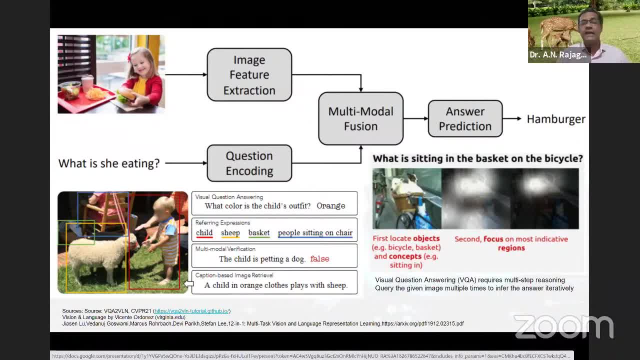 or you could play some attention mechanism, whatever it is right, I mean, it's entirely up to you- And then eventually you post it as a classification problem, right Where, at the output? right, You say whether it is hamburger. 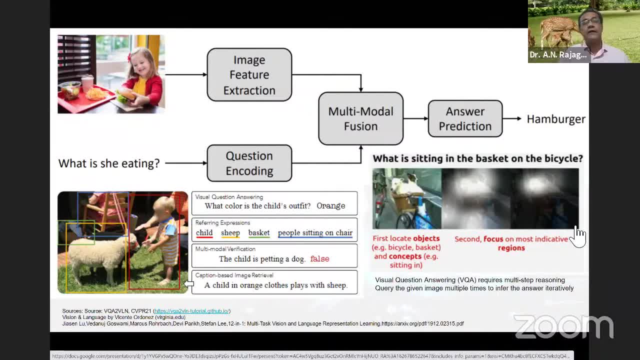 whether it is something else, and so on. right, You could also go one step further, and then you could also talk about a multimodal verification problem, As they say right. For example, in this left picture that you see here, I mean, you see a kid next to a dog. 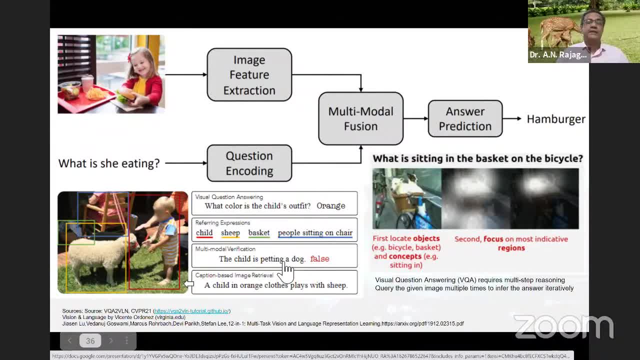 and apparently you can ask the sentence: is this child actually petting a dog? And then you can answer with a false or true, And in this case, of course, it's false, And you can go one step further. right, You can also look at problems that can use a caption. 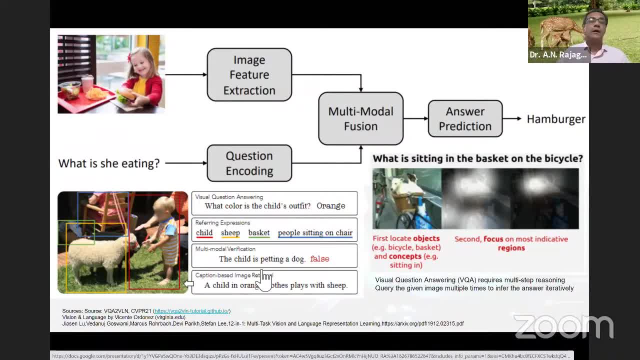 in order to be able to retrieve an image right. For example, if I wanted an image like this to come up, I could ask and I could kind of throw in a sentence like this, which says: a child in orange clothes plays with sheep. 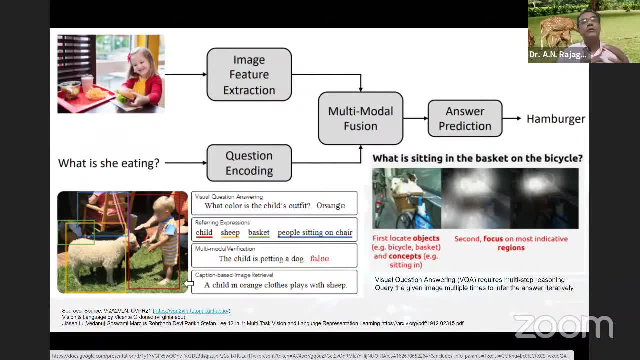 Now just try to bring out all those images right Which look like that. Now again, a framework like this requires you to marry the features right That come from text and then to what you see right. So in this case, it's the image feature. 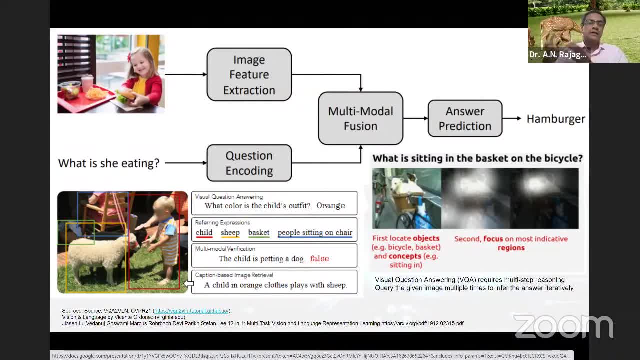 So normally what is done is a nonlinear mapping- right, It's learned- and then try to marry these two features And therefore, right during a test time and when you kind of input a sentence, then that same kind of a nonlinear mapping. 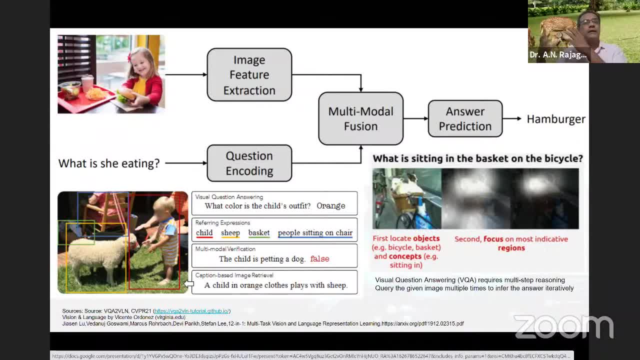 which has been learned through several examples, is then brought on, and then it is applied on your sentence, And then it finds out with respect to which visual feature you know: is this, is this, is this kind of close right? Is this: is this, is this kind of close right? 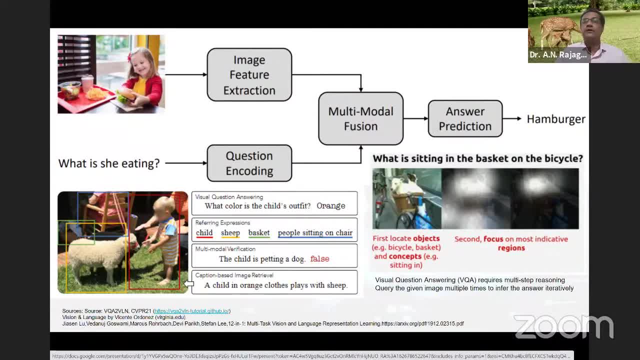 Is this, is this, is this kind of closest, And then whatever is the image with respect to that you know is basically shown to you right? Let me kind of go back and I also wanted to talk about another one. 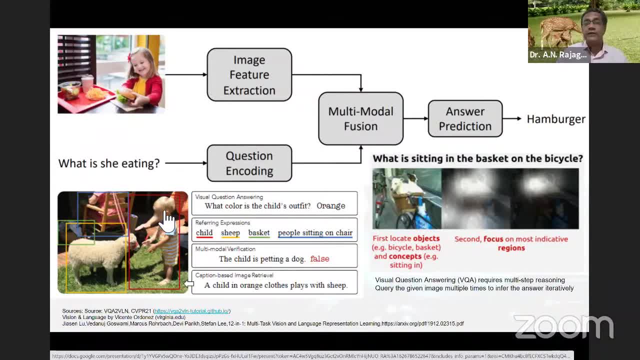 You can go one step further. There are works that talk about you know, a text to picture. So here, right, somebody just writes up a text, and it's not about searching for an image, It's about, you know, having a deep network. 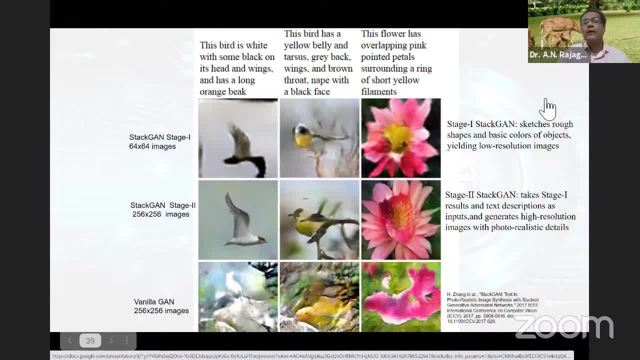 generate the picture of a certain kind. Now, you know most recent work, right, which came in 27,. not very recent, but a 2017 work talks about, you know, having two GANs. you know they call it stack GANs, right. 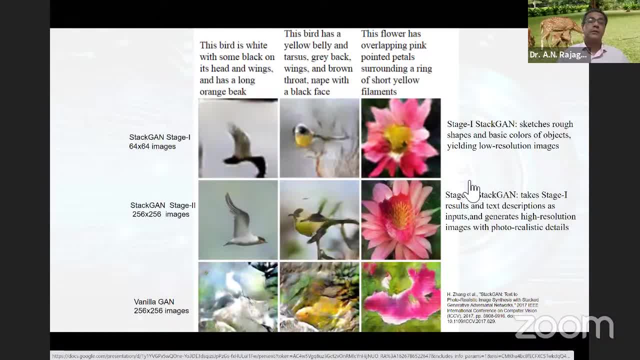 You know they call it stack GANs. right, You know they call it stack GAN one and a stack. you know stage two and stage one and stage two, But in stage one when you get a rough idea. 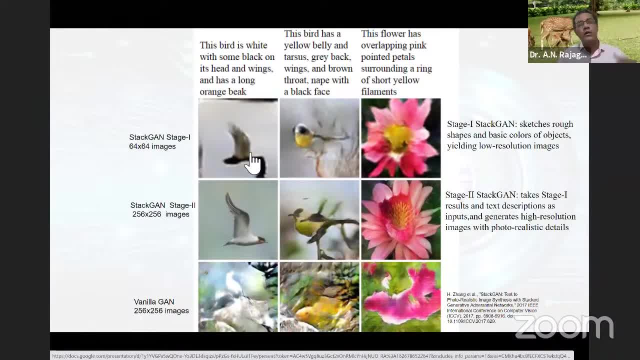 about what is being asked and then in stage two, right, you use again, you go back to your text and then go back to this visual picture that your stage one has been able to reconstruct and then use that to actually refine your output. 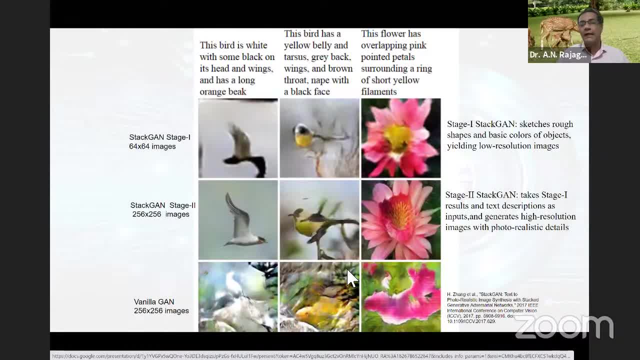 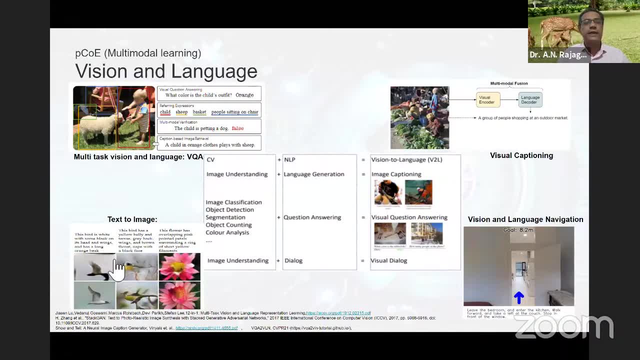 Then you could also do a visual dialogue right, And you could also do a grounding right. I mean a visual grounding, So I'm going to play this video- and where you see that you know, for a navigation task. 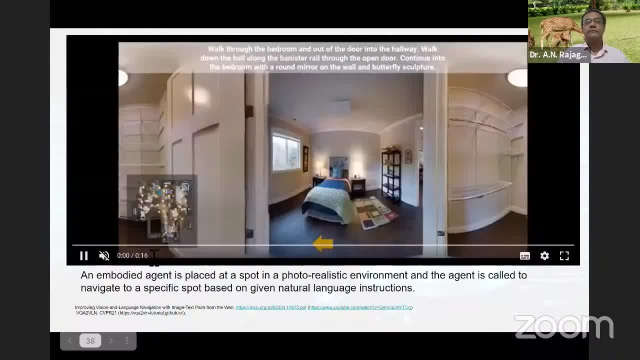 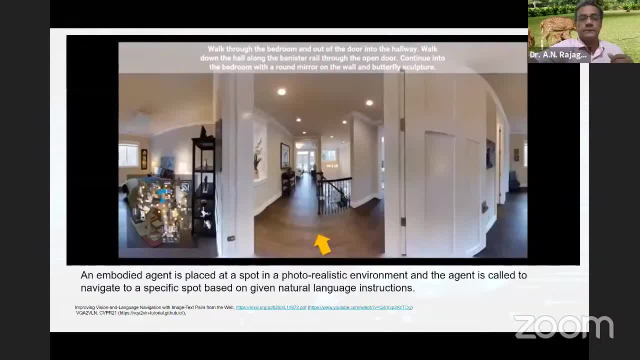 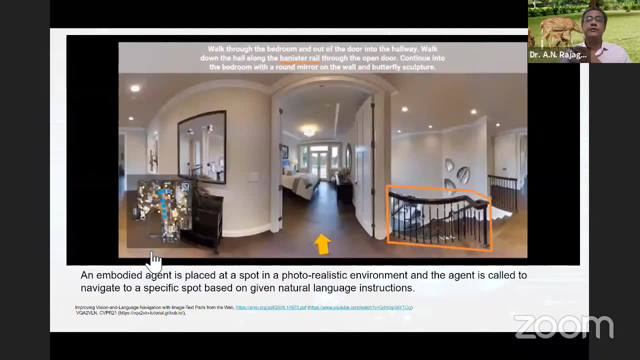 Language navigation instructions. as shown on the top, A key to solving this task is grounding visual concepts mentioned in the instruction, such as banister rail and the round mirror and butterfly sculpture. Prior work. So you saw that. so you saw that as the 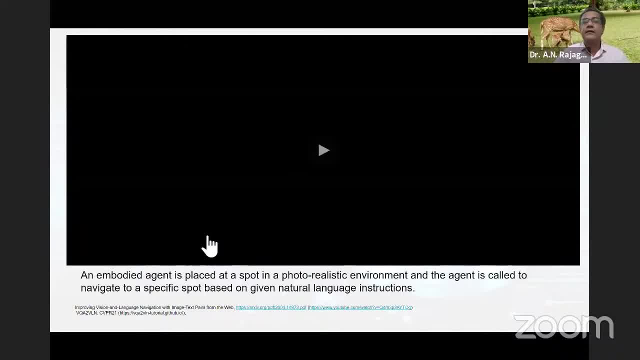 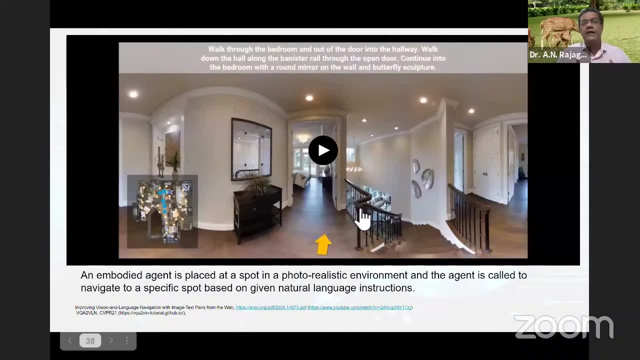 as it kind of goes through the text, right, It realizes that you know that there is a banister, which means that it has to visually ground the text. So this is something like an embodied agent, right, Which wants to navigate from, let's say, point A to point B. 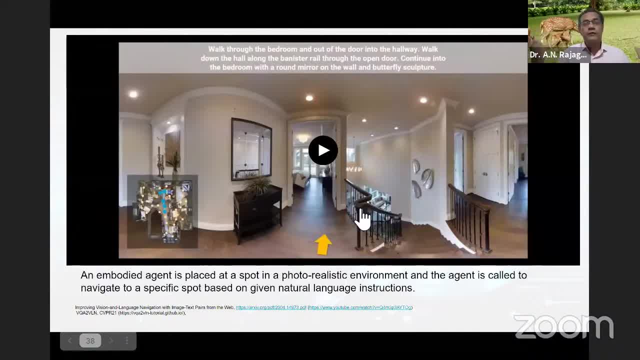 Then along the way, instead of just seeing what is around, and if you could also kind of guide it through a textual sort of information where, in this case, it is able to ground what you're telling. there's a banister, and then right, and then along the way. 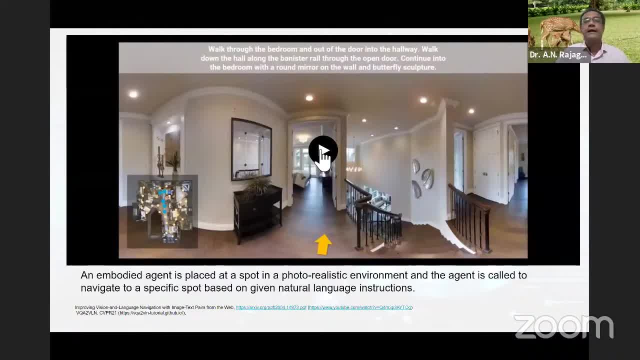 it also said that there was a round mirror right And then right, I think it also said about, talked about a ground mirror, a round mirror, and then there was a butterfly structure and so on. So if it is able to ground all of that, 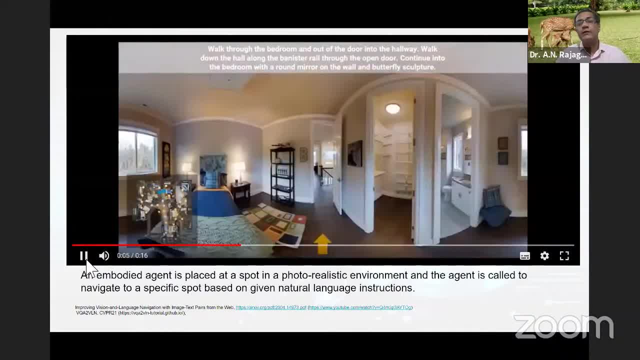 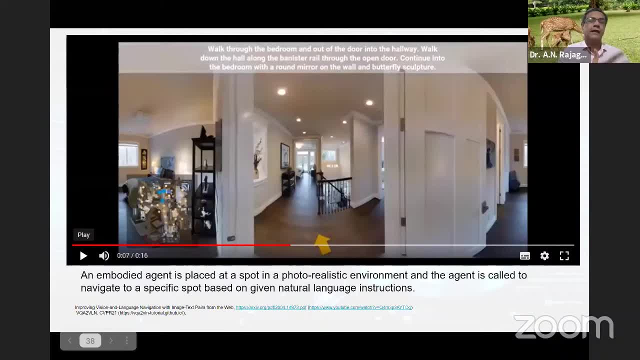 then you know it helps. it helps it navigate right From, let's say, point A to point B. okay, Moving on, you can also combine, of course. you know audio right. I mean when you have, when you have images. 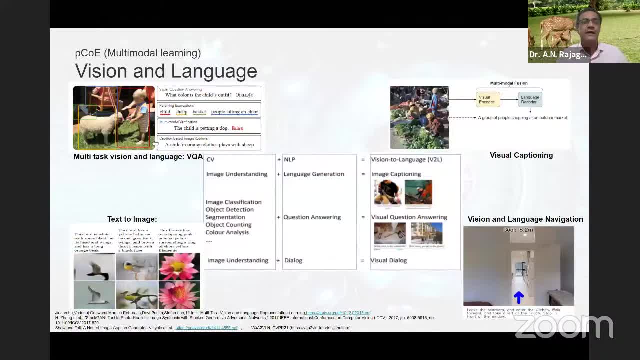 you can also combine them with audio, right, in order to solve some very novel tasks. One of the first ones right- I don't know which I intend to talk about- is really, you know, creating, creating a stereo, or kind of what is called. 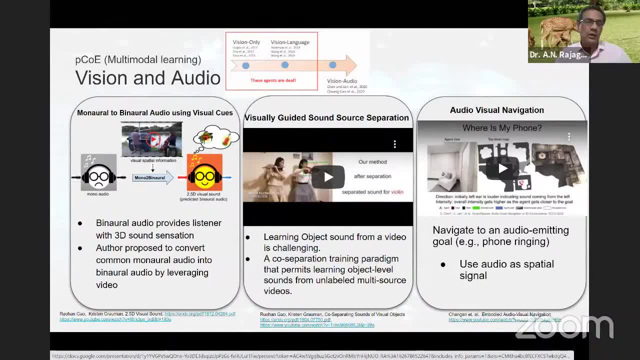 a binaural audio from a, from a single channel audio which is a monaural. you know that is a monaural audio. A monaural is like a mixture of left and right channels And I know it's an important problem, you know. 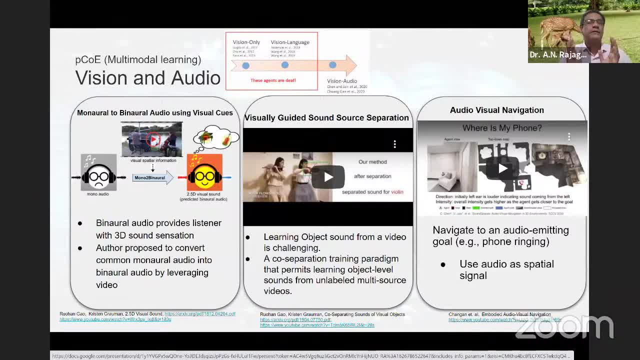 it's because it's very hard to create a stereo setup that would actually emulate your head sort of a transfer function. right, Because our head is. you know, head has a certain sort of a construct and it's not often that right. 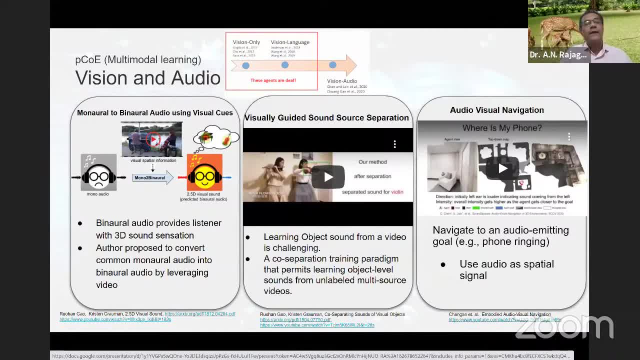 that these people keep speakers that way or keep these mics that way, right? Therefore, one of the one of the nice things is is being able to convert a monaural audio into a binaural or a stereo output. 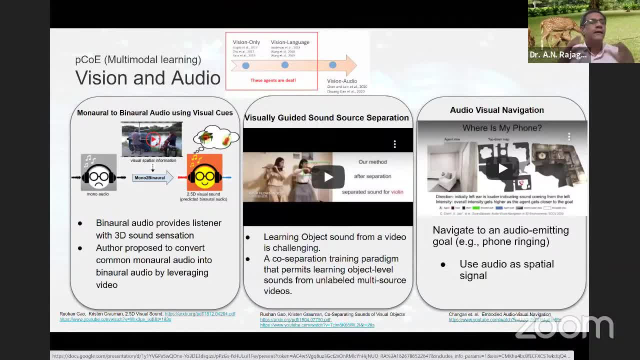 because with a stereo output right, you get a sense for where the objects are. right. I mean, even if you don't see the image, you get a get a sense for something being on the left and something being on the right, and so on. 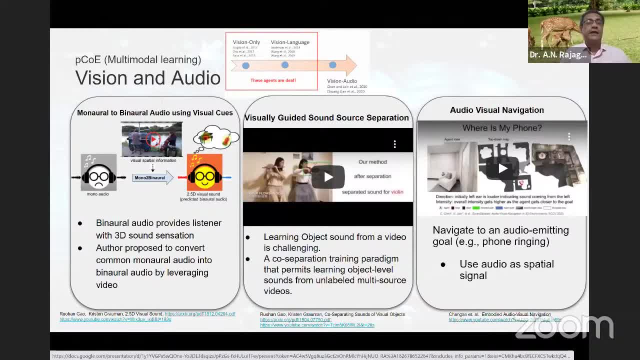 that gives you a spatial cue. And then images are fantastic in that sense. right, Images carry a very strong spatial cue and right, which is why it's got- something like this would actually exploit. So right, I'm going to just play this. 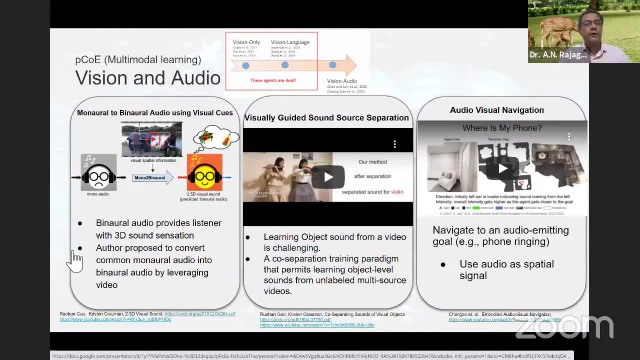 play this video for you And if you've got a okay right, let me just pause for a moment and tell you that if you have a headphone on and you will be able to see that when the car is on the left right, 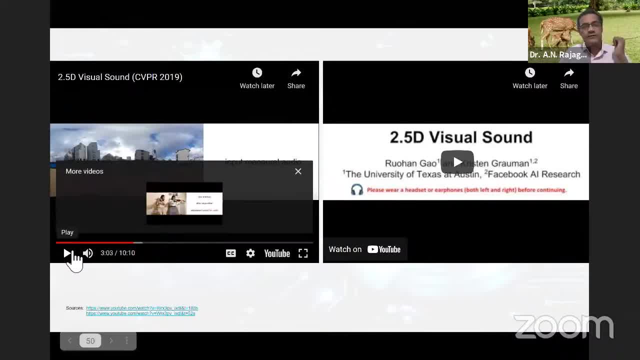 that you'll be able to hear, hear, you know sort of you know sort of a dominant sound in your left, left, this one headphone and then, as the car veers, and then, you know, takes a U-turn and goes the other way. 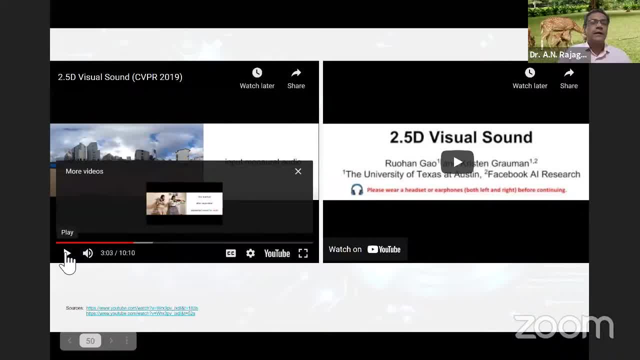 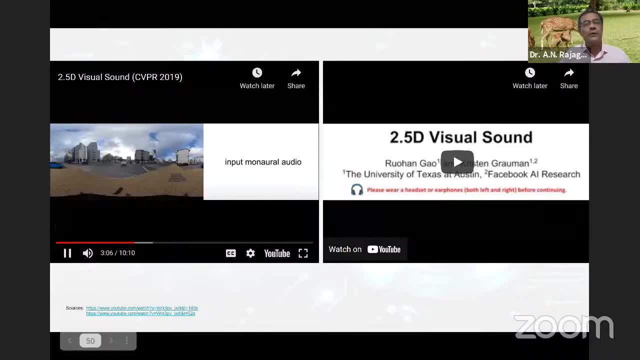 you should be able to see a shift right in terms of what you get here. Okay, now I'm going to just play this. This is the monaural audio. Okay, this is the monaural audio. There's no stereo. 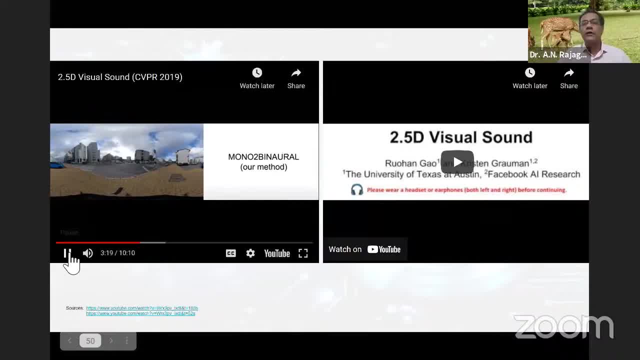 Now. so this is binaural right. If you had your headphones on, you will be able to right. you would have been able to see that. Now here is another, here is some instrument, right? So these people have been 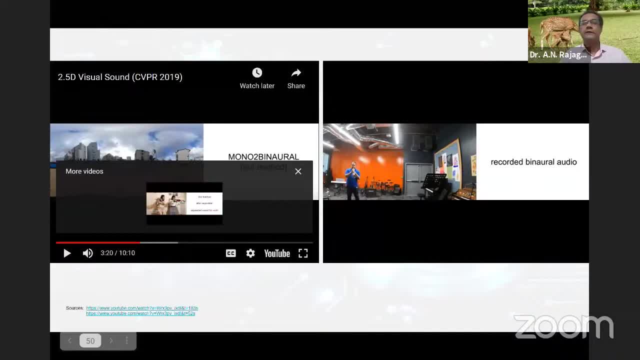 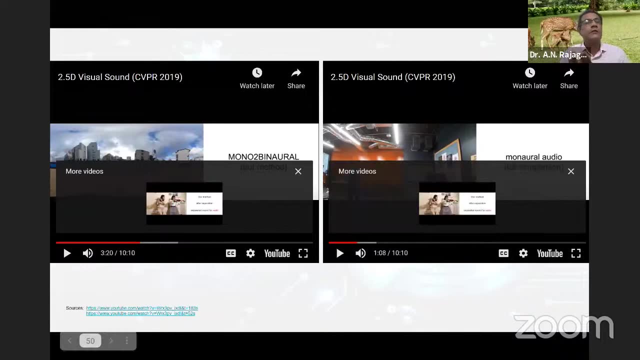 Okay. so in this case, if you're wondering, why would they want to do it if there is just, you know, one instrument? you can also do it if they have your multiple instruments. but then even with one instrument, you want to get a sense for from where it is being played, right? 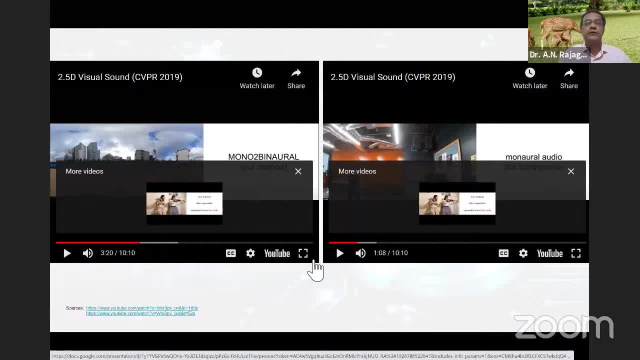 and therefore you know it's important, even for such right, for such a problem, You can actually go one step further and then you can talk about. you know, talk about locating, or you know, do do the sound source. 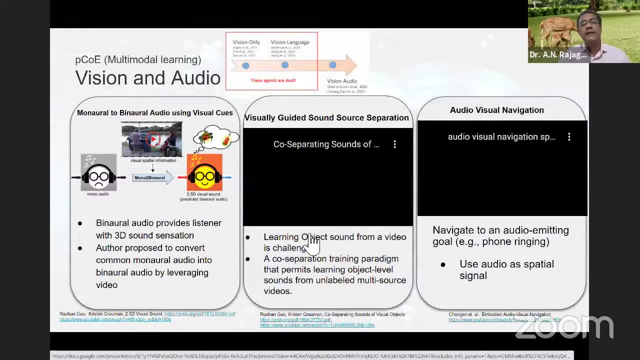 a kind of a separation right And for that, and I'm going to play this video, and the nice thing about the second one is that you know there are no. I mean you don't have really a kind of a ground truth right. 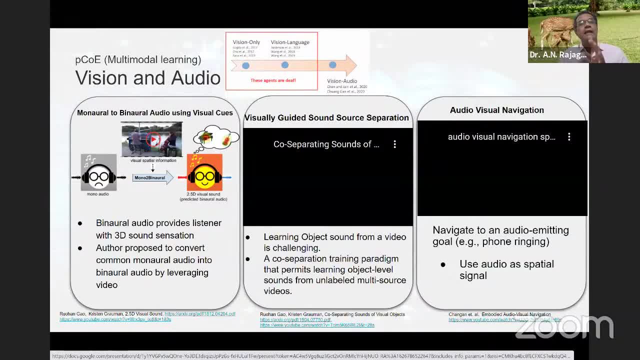 Because in most of these right you don't have, you don't have ground truth labels, and yet you have some kind of a weak supervision going on which helps you, which helps you to, helps you to, kind of see, do this. 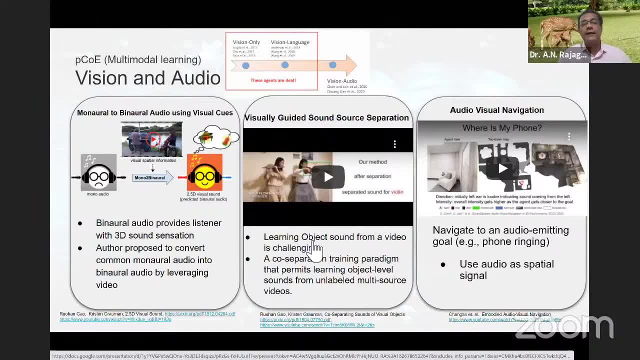 Now I'm going to play this video first, so that you get a sense of what is what is happening, and then I'll kind of see, come back and come back and, right, talk about, talk about, right, what it is. 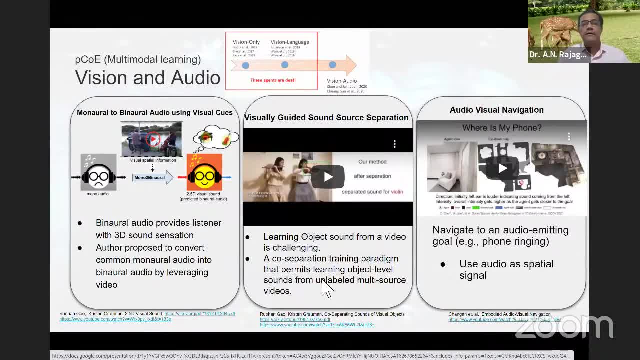 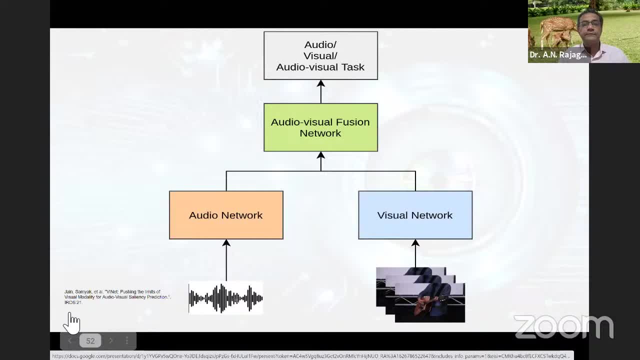 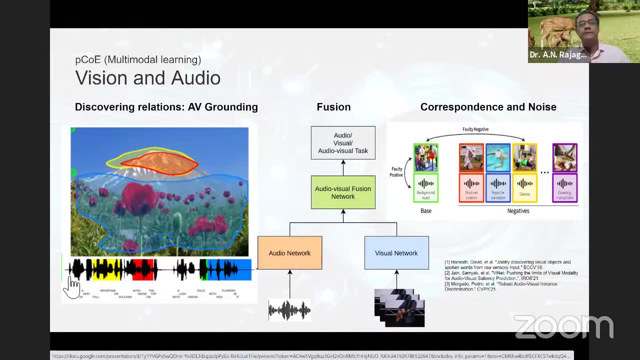 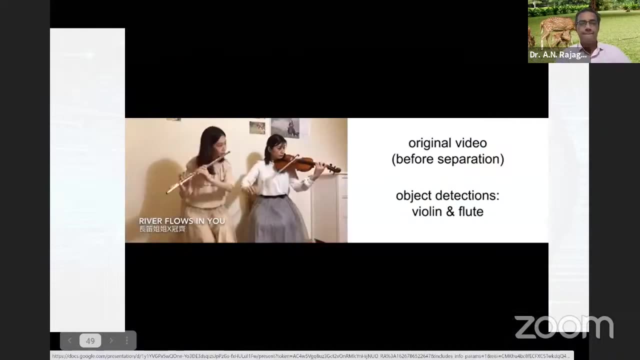 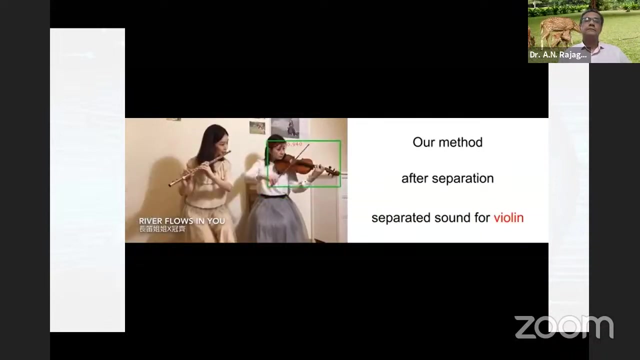 Sorry, let me go back one minute. Oh, oh, let me go to the previous slide. Yeah, here, Okay now, okay now if you, if you actually hear right, there are these two people. Yeah, so so you could see that you know there was. 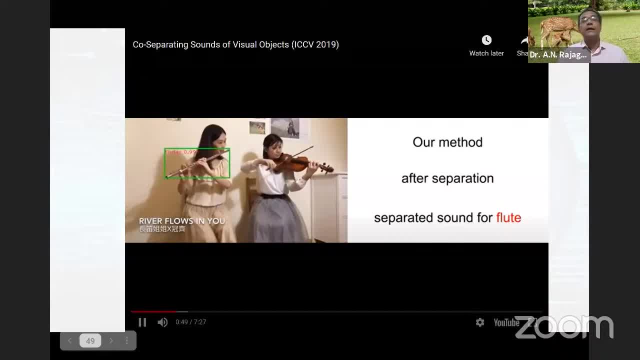 there was a sound source separation, right. that was clearly happening, right. So so, on the one hand, you could, you could just hear to violin, or I mean, if you chose to, just, you know, hear to the flute, right. 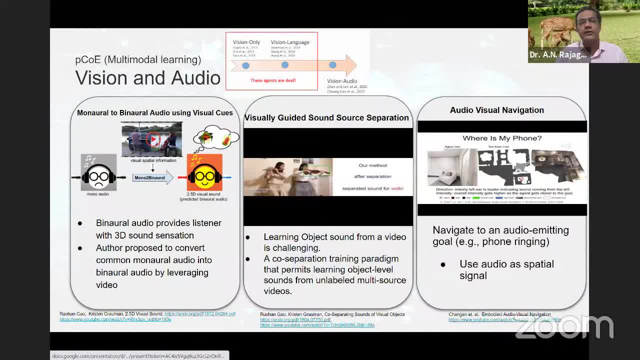 you could do that and and all of this with some, with some very, very weak supervision, right, in the sense that here, here, you know, the kind of visual cue is simply the fact that, right, you've seen certain objects, right. 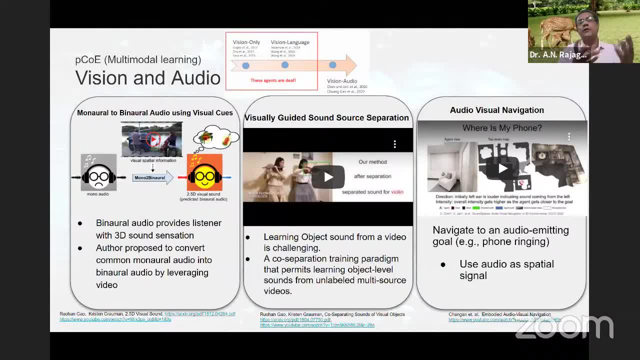 So, in the sense that you know you've seen a flute- I mean which, which you know, which, of course you can have deep networks- they can tell you that you have a flute in the scene, you can have right. I mean you can, you can even know that. 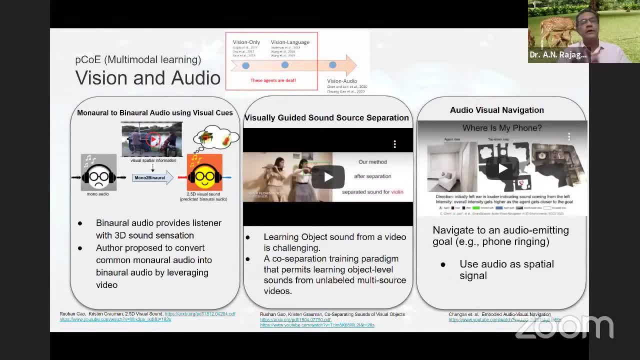 there is a violin in the scene and so on, and this and this works on the fact that there's a kind of a co-separation, and which happens. co-separation is very similar to this kind of a co-segmentation. 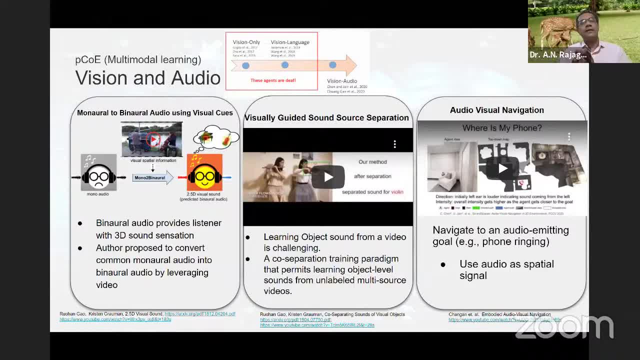 right, which we're, which we're all familiar with. but here the co-separation is something like you kind of mix two, right, mix, a video one and video two, and then at the output, you expect, right, each of those, each of those audios to emerge. 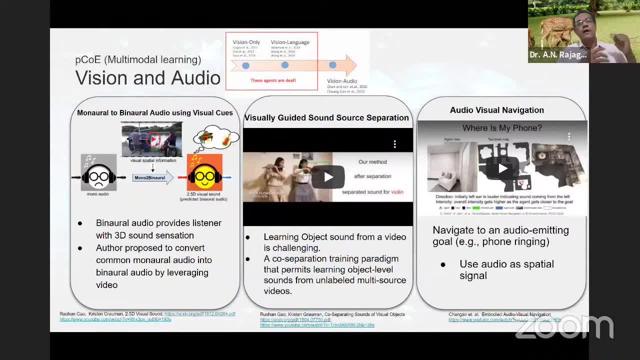 but at the same time right. the image cue comes in the form that you expect, that you know if, let's say, you know if in two videos you saw, you saw, you saw the same instrument, right. 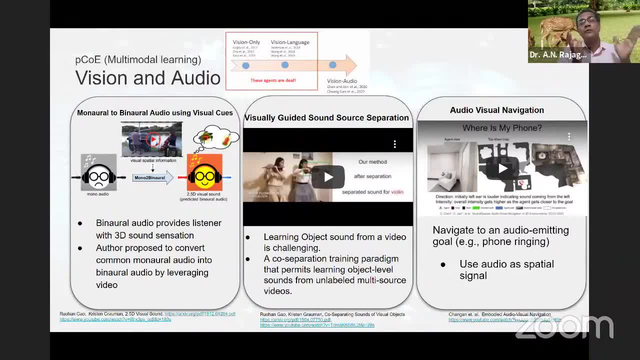 and they said that you know, both are, let's say, flute or something. then you expect the sounds to also be close, right? that is the only supervision that it really uses. so you know, there's no, there's no, there's no very hard supervision, right. 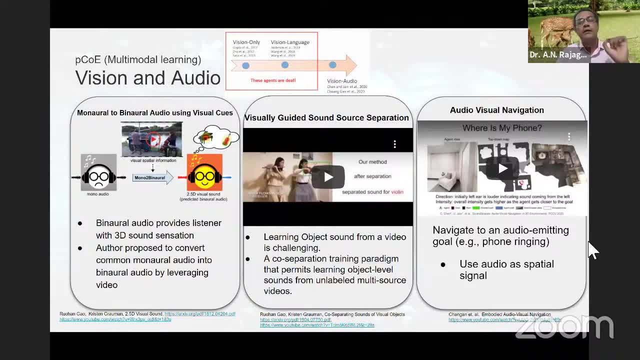 which is actually going on, and with just that right I mean, you're able to achieve something like that: Raju, you have five minutes, Yeah, and then, and then, of course, right, I mean, you can also do some kind of a grounding right, which means that 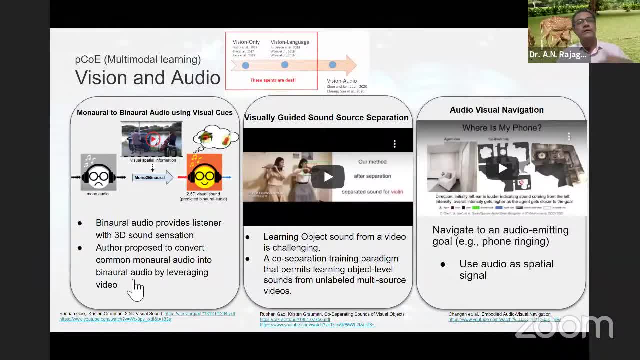 you can have the speech out here, right, I mean? and then, while, while somebody Right speaking, you might want to relate as to what in the image right does this kind of correspond to. so, for example, right, the red one. 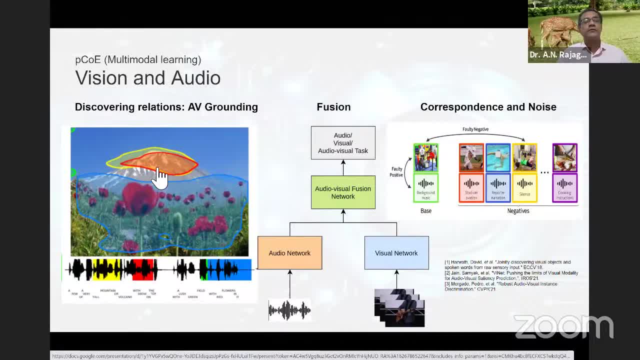 the red one is about, you know, snow on the top right, which is what is being, is being shown here, and then this blue thing is about flowers with a red. you know, the red flowers right and so on, inside a garden. 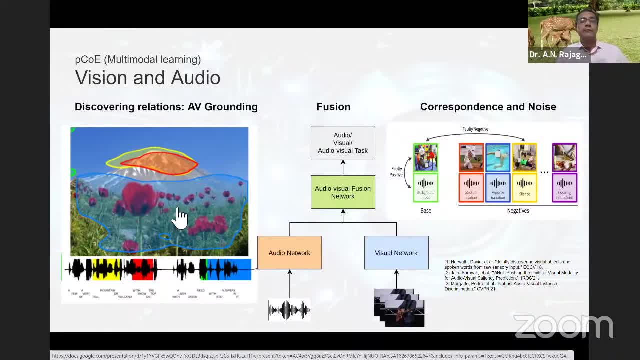 and then this visual grounding right is also a very nice problem, can be used for video parsing and so on. but then it's not true that all is hunky-dory right, because what can happen is, you know, many of these labels are very weak, or many of these labels are noisy. 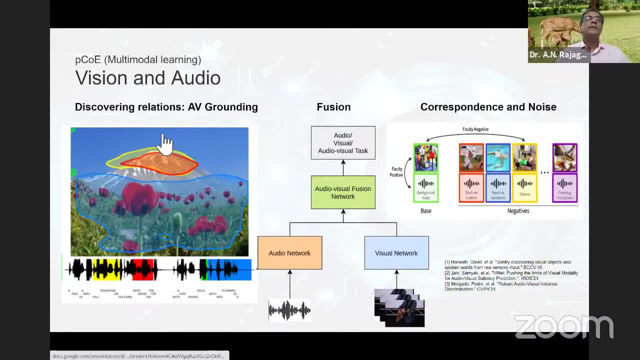 for example. right, I mean, you know, here is a situation where, let's say, somebody, somebody you know, says that here's the right label for a weightlifting and here it's background music, which is actually a positive. 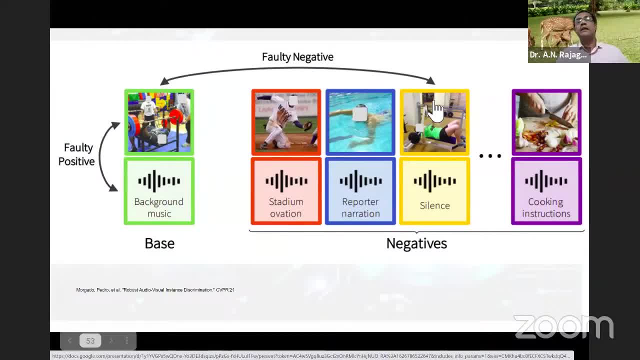 which is a faulty positive. okay. so therefore, what can happen is a similar weightlifting. otherwise, what will be a true positive is silence. now, what happens is when you actually mix up labels like that, which is not in your hand and really you don't know which one is correct. 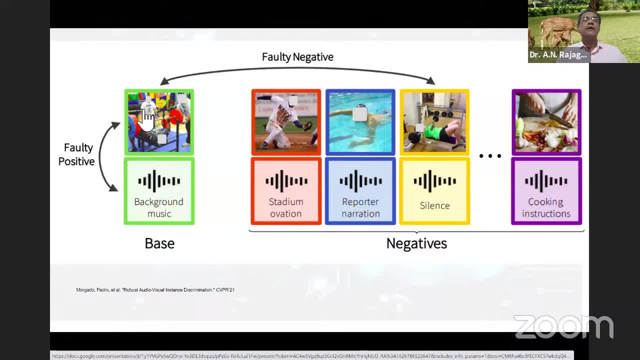 and therefore, in such a case, what can happen is this can become a faulty. when you do kind of a contrastive learning right, this could become a faulty negative for this guy and this background music could be a faulty, a faulty kind of a negative. 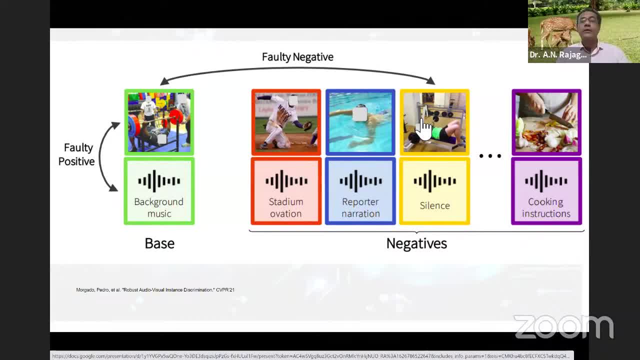 you know, for the, for the, for the right, for the other one. okay, so, so in that sense that all is not hunky-dory, so we have a long way to go right and and then right going forward. 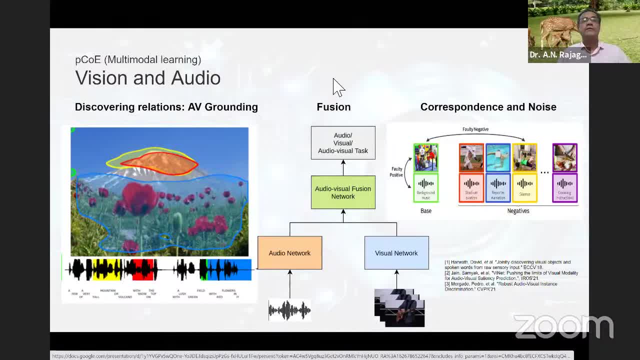 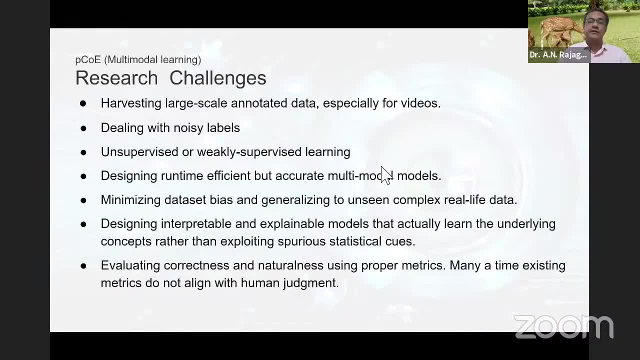 so the vision challenges are many right. I mean, as I said, you have to harvest large-scale annotated data to deal with noisy labels, unsupervised and weakly supervised, learning, design, runtime, efficient, multimodal, multi right, multimodal models. 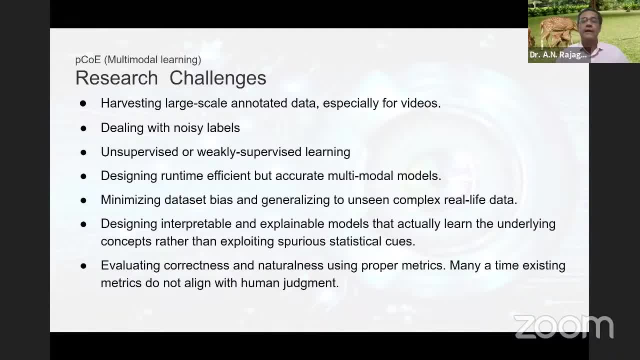 and then interpretable and explainable models- right is what you're looking for, and so on. and even the metrics are not really very clear. they don't seem to align very well with our human sort of adjustment. Then, moving on, we also want- I also wanted to talk about this other area- 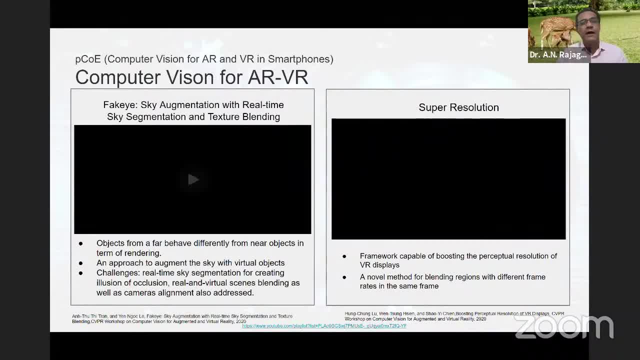 it's about computer vision for AR and VR, mainly from a smartphone kind of point of view. so, for example, right, I mean you could have something like this, where where, as you drive through a road, right, you want to. 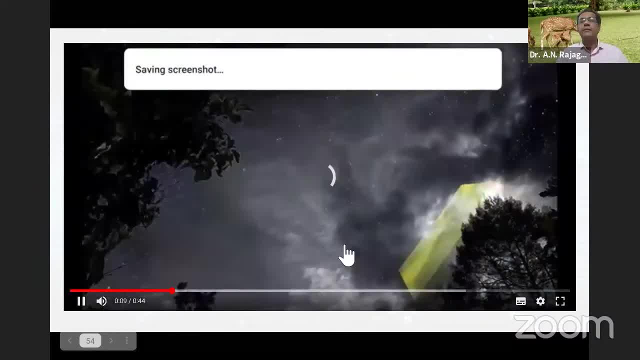 you want to. you want to, sort of- right you know, bring in something into the scene, something like this, right, so here is the natural scene, and you sort of insert an object right into the scene in order to just simply enhance a viewer's experience. 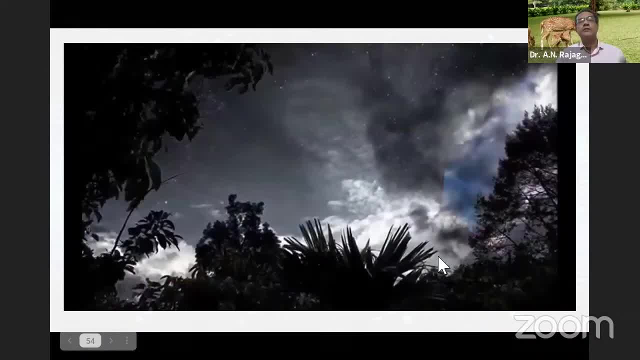 it could be that, or, or, for example, it could also be super resolution where it is gaze-driven, for example. if you're interested in this area, that is what you know brings up, that is what gets super resolved. 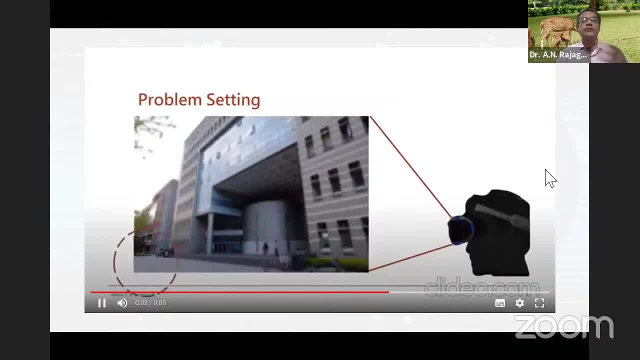 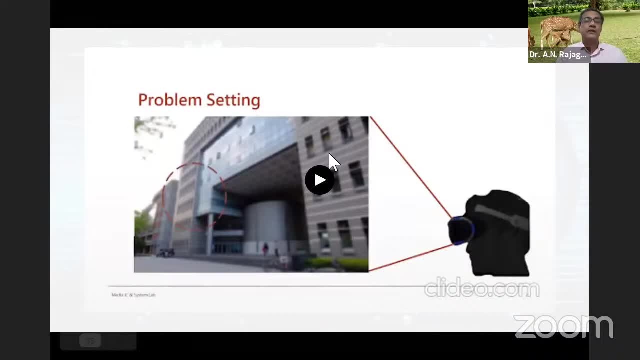 or you keep moving your gaze and then and then you want to be able to super, resolve things of interest. right, these are again things you know which you can do on a smartphone, but then, as far as the, as far as our own research, 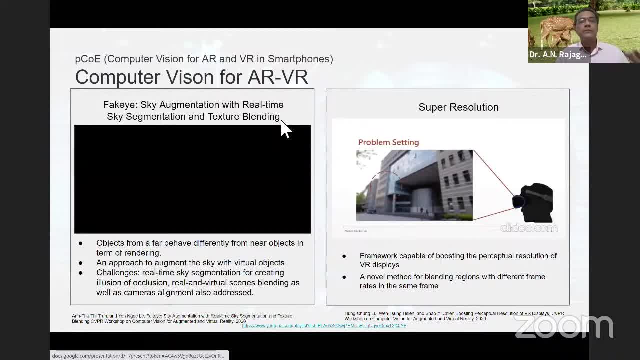 you know sort of you know path ahead is concerned, and we, we are more interested in doing this for this, for